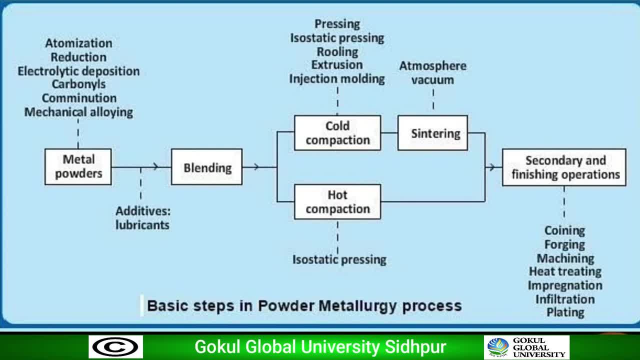 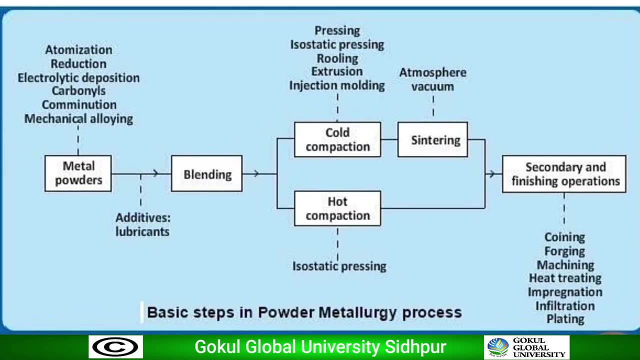 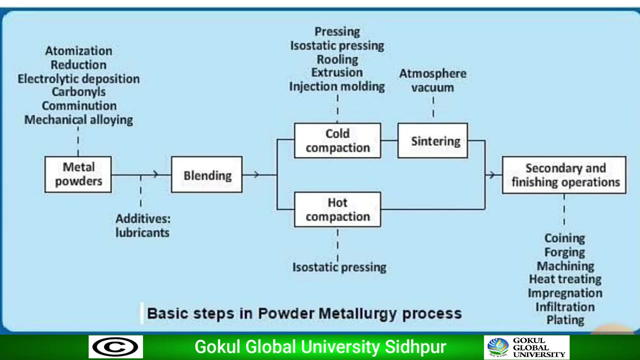 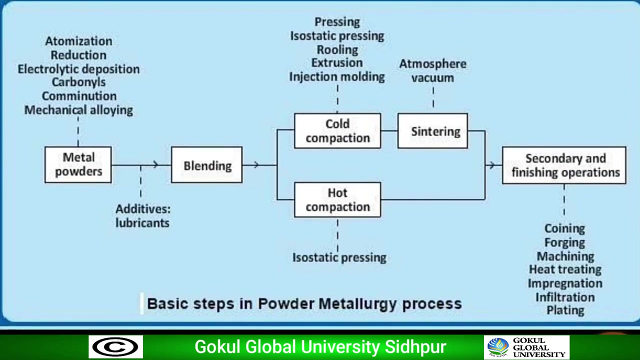 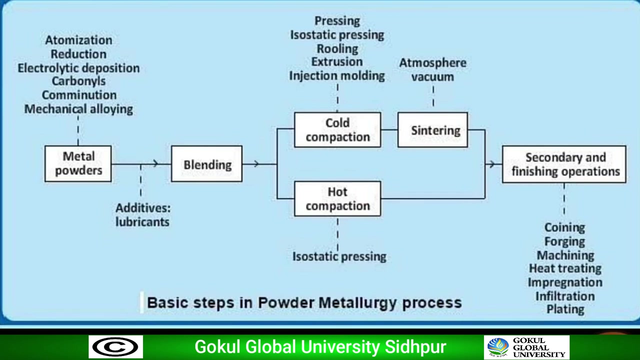 one is atomizations, reductions, electrolyte, mechanical allowing, Then next blending process. Blending is the meaning of one types of mixing process. Now, blending process, Blending is the one types of mixing process. There are two types of compactions. Compaction is the one type of pressing operations like that hard compactions. 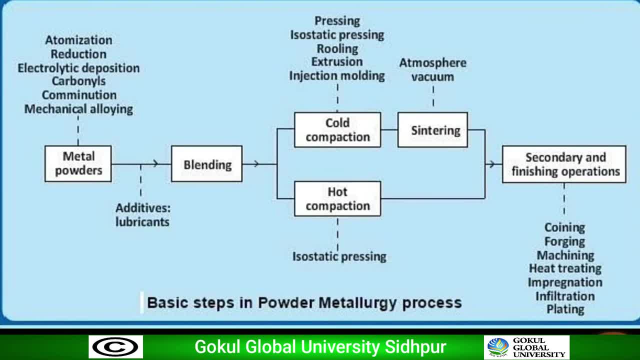 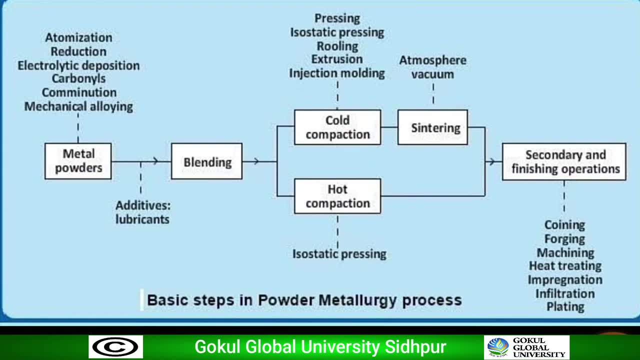 and cold compactions-. HOT COMPACTIONS means it is the defined as the material needs elongate above recrystallizations boundary and cold complexions. it is the defined as a material can be below recrystallizations temperatures. it's a. 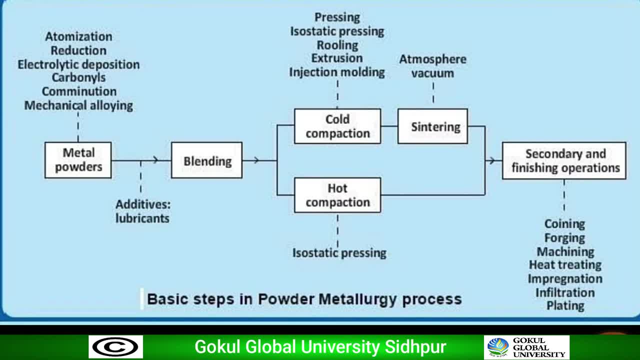 like that: pressing, isostatic pressing, rolling, accidents, injection, molding. okay, then now product is converted into sintering process. sintering it's like that, pressurize of atmosphere, vacuum systems. there are two types of sintering process. first one is solid types and liquid types in this materials. first one: 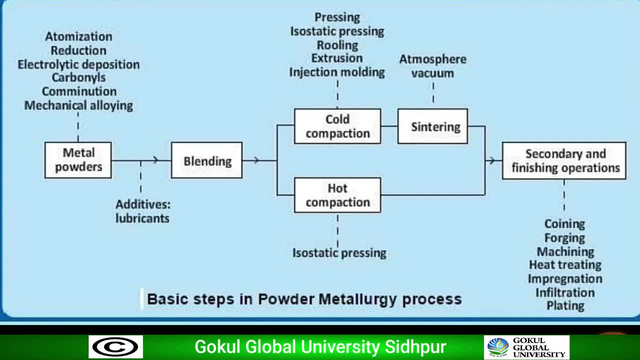 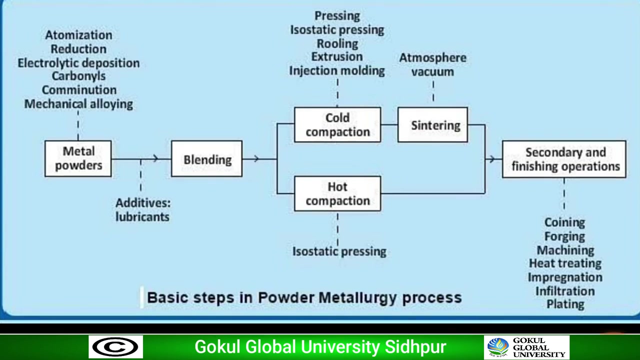 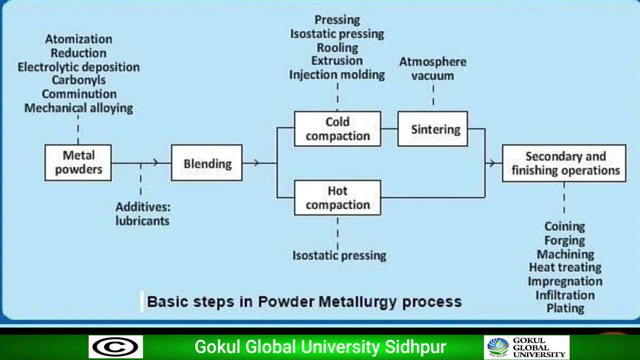 are discussed about solid types sintering process in this body. in this process the material can be enter and quenching process above recrystallizations the metals can be destroyed. particles discuss about a liquid phase in this materials systems. sintering systems can be provided below recrystallizations and their bill phases. 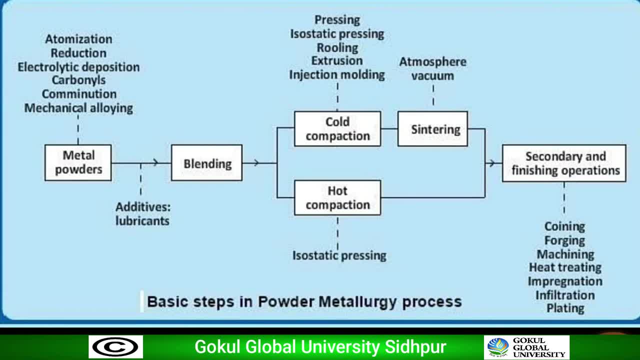 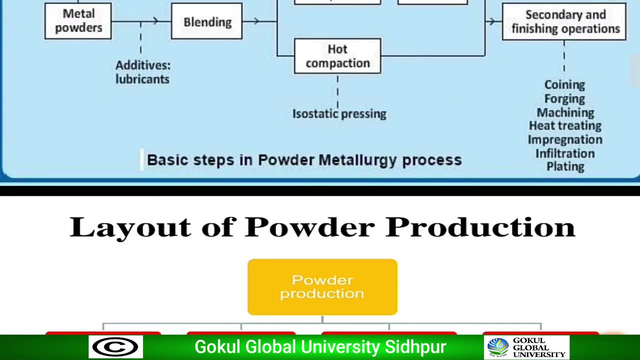 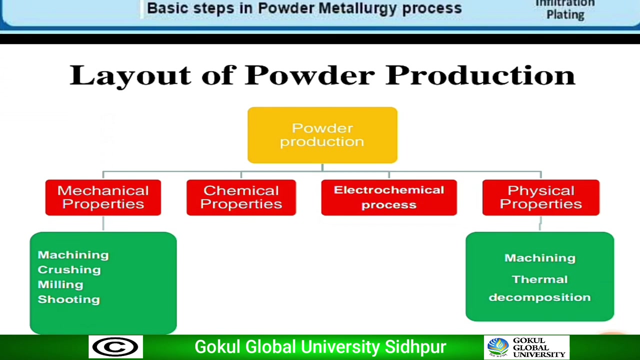 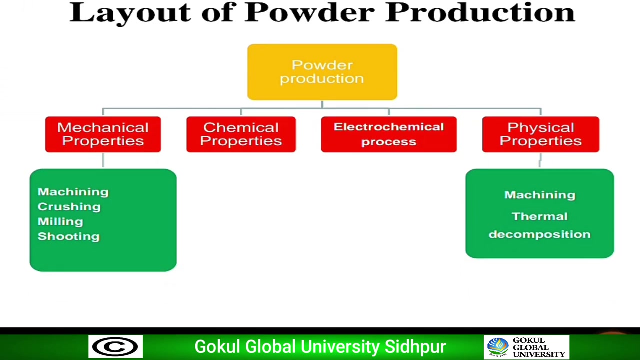 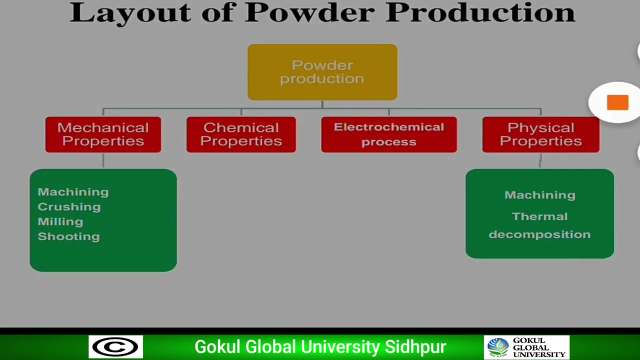 can change. then it's convert into secondary parts, operation like at quenching, forging, machining, heat treating, integrations. let's discuss about a layout of powder production. now four types of properties: mechanical properties, chemical properties, electrochemical properties properties: now let's discuss about a machining process. in these mechanical properties. first one discuss about machining process. 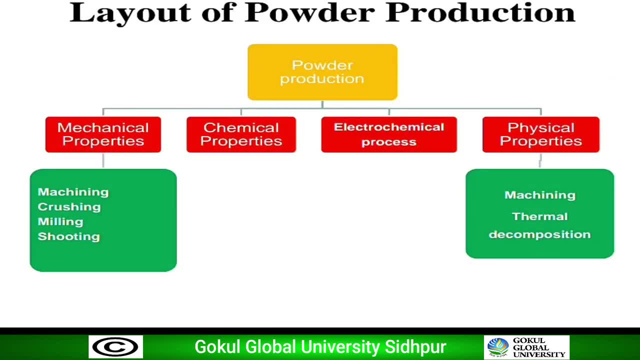 now friends discuss of the machining process topic and why, or the over the, the overporte process body我在 now friends discuss of the overporte process body ubiquity problem. now friend discuss over the overporte process machining process. a principle of the chips so obtained are broken by. 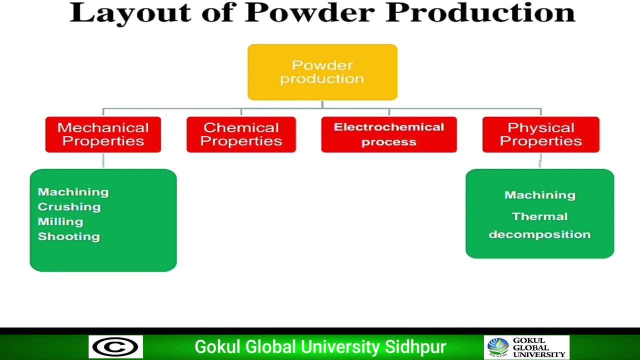 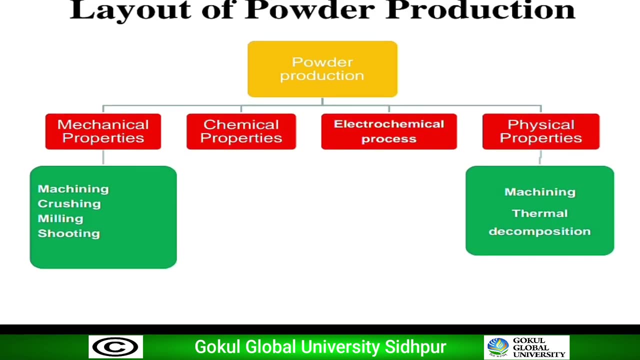 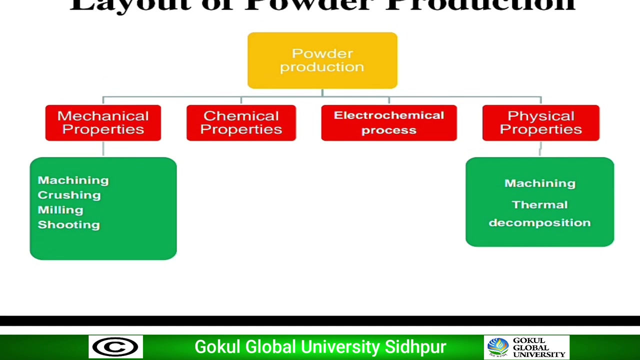 subsequent crushing and milling. then applications of like that: dental alloys, chromium powders for tracer bullets in defense, applications like that. second properties: crushing. crushing is the. in this method, the small pieces of the materials are collected and crushed together. breeder materials are most suitable for crushing techniques and producing irregular safe particles. 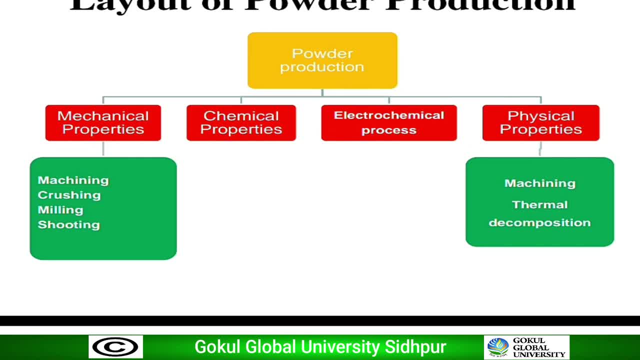 octal materials get elongated before fracturing and their powders are flaky in shape. now discuss about. now discuss about the chemical properties. now, friend, discuss about a chemical properties. first. one is reduction, reductions. matter is based on the principle of breaking the oxides oxalate formats in this method. 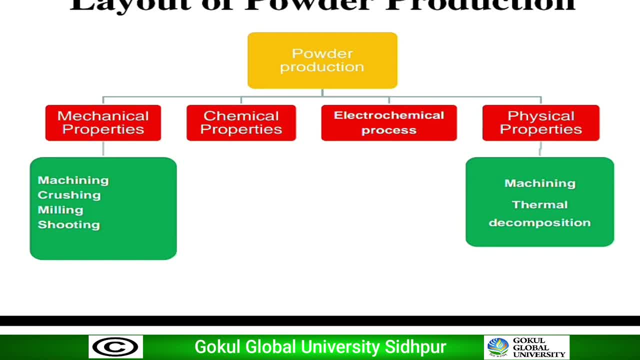 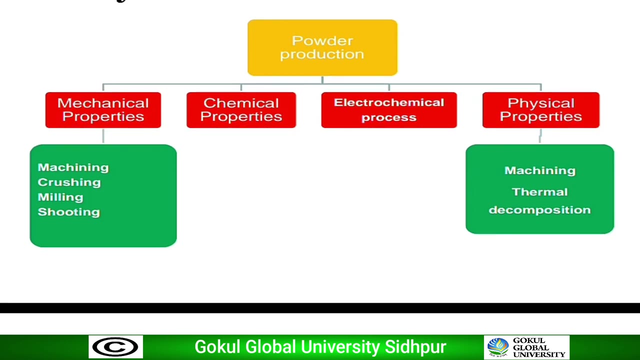 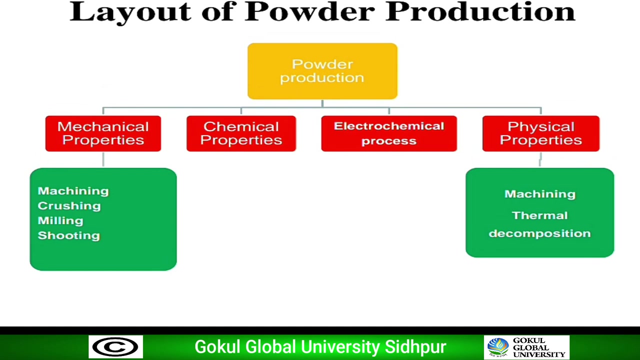 economical and flexible in use now any yä underscore chemical process which can be used for various types of mechanical products. that which can be used for various type mechanical products for various type metal powders are obtained by cutting the touched into around the prisoners, along by electro depositions from their metal. solutions are foods, salt, like that. 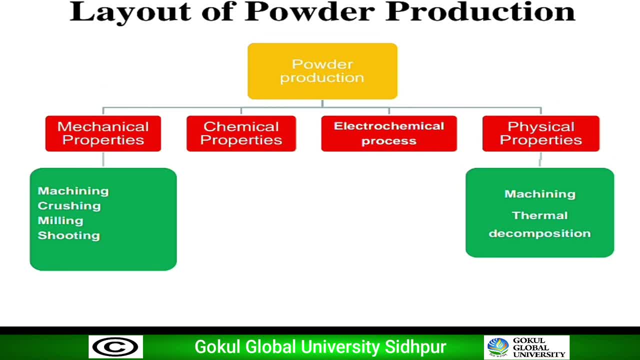 depositions as hard and brittle mats, which is the further crust to produce powder. depositions as soft and spongy substance, loosely hydrant, which is the further powder by rubbing. okay, now discuss about a physical properties. now physic physical properties. first one is condensation. condensation is the 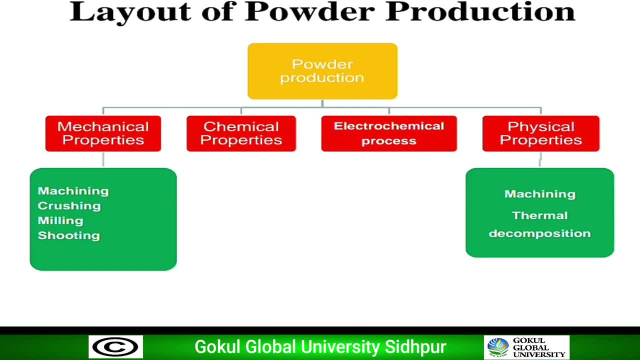 operation of many types of metals converting to vapors obtained by metal powders. it is suitable for volatile metals that get easily transformed into vapors. then second one is thermal decompositions. now, what is the meaning of thermal decomposition? this method amplifies the principle of decompositions. the carbonyl. 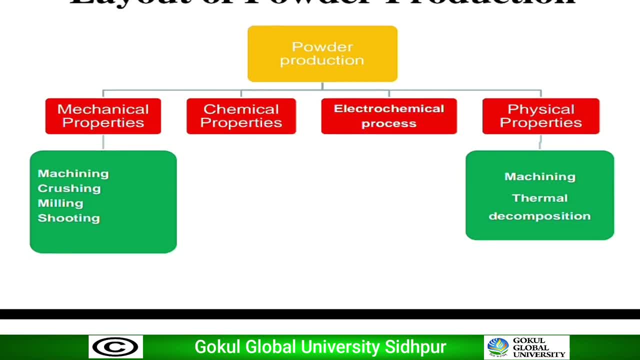 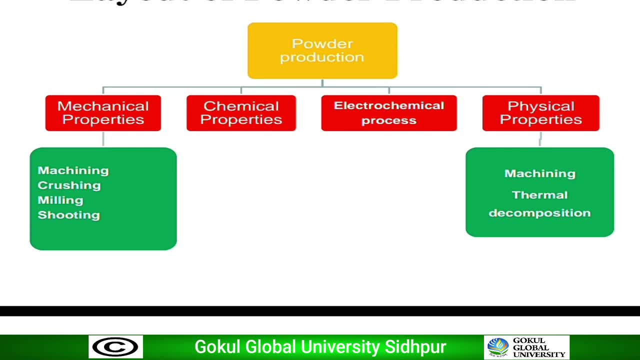 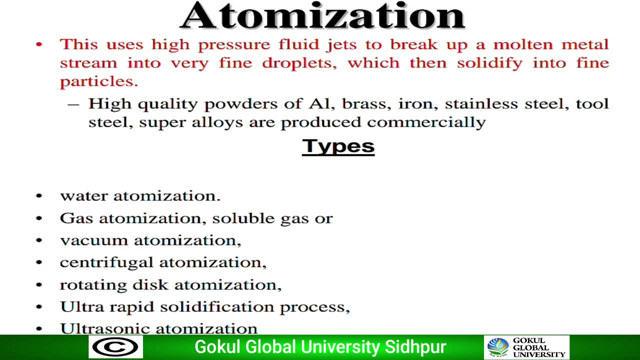 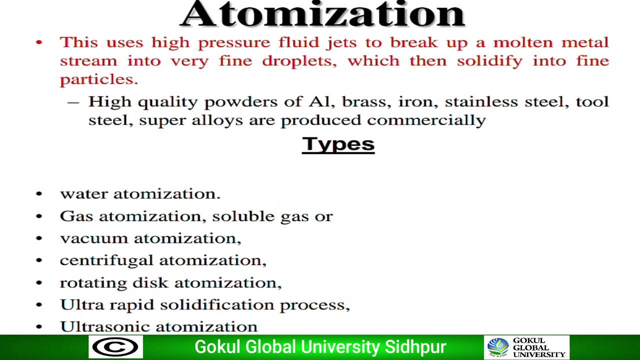 vapors of metals at control temperature and pressure conditions and breaking in the metal into powder. now, now we'll discuss about atomizations. now, what is the meaning of atomizations? these use high pressure Dis瑕's to break up Moulton metals stream into very 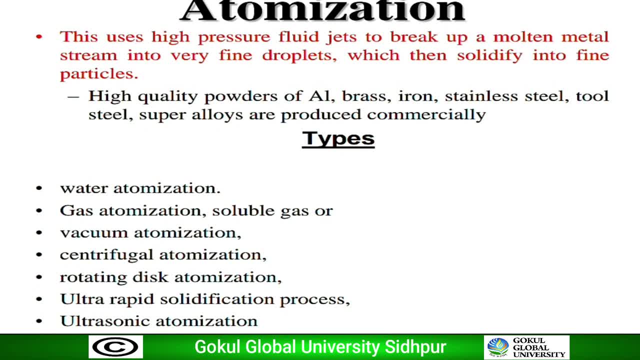 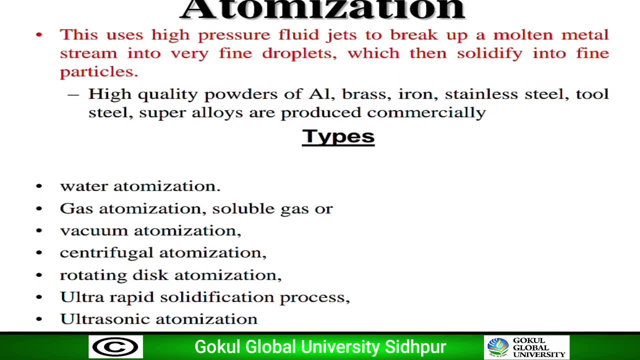 fine droplets which the solidified into fine particles, inasallas methods of personalization and toxic batches high-quality powders. Transocolmia is using burlqouq and the answer to a carbon can be any chemical. softز of aluminum, brass, iron, stainless steels, steel stools, super alloys are produced. 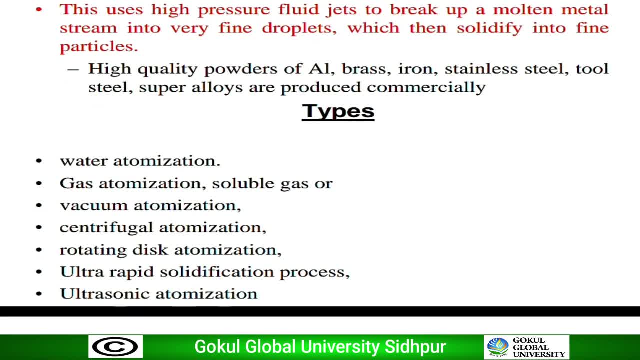 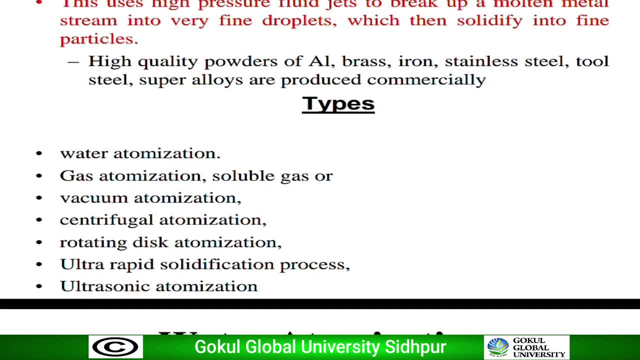 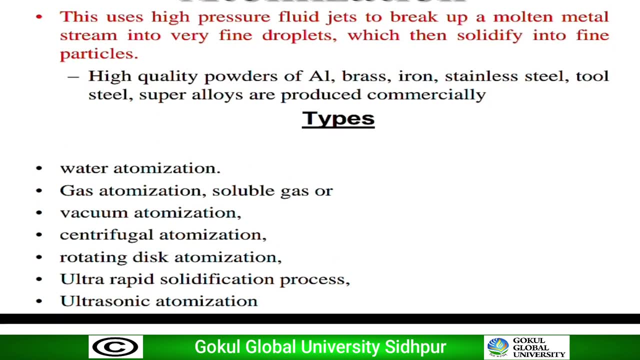 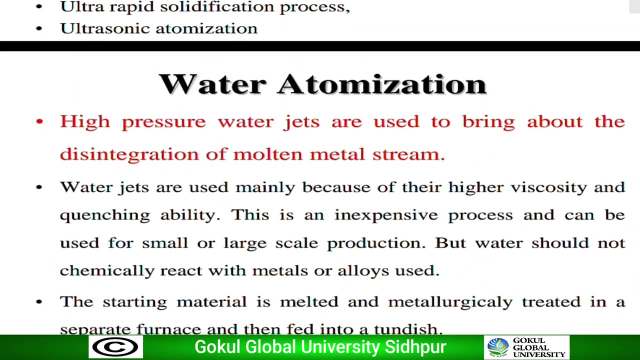 commonly used. there are lots of types of atomizations process. now first one is water atomizations, gas atomizations, vacuum atomizations, centrifugal atomizations, rotating disk atomizations, ultrasonic atomizations. now friends discuss about water atomizations process. high-pressure water jets are used to 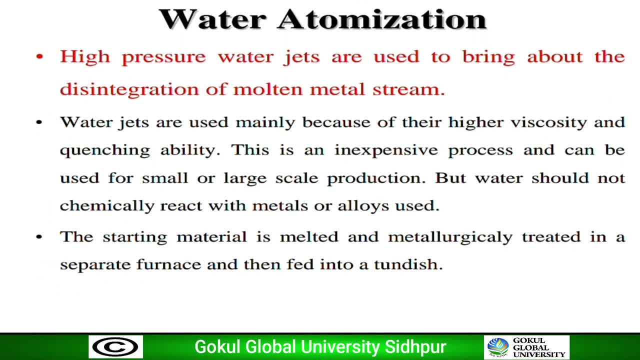 bring about the distinctions of molten metal stream now a water jets are used mainly because of their highly viscosity and quenching ability. this is an inexpensive process and can be used for small and large scale production, but water should not chemically react with metals or alloys. 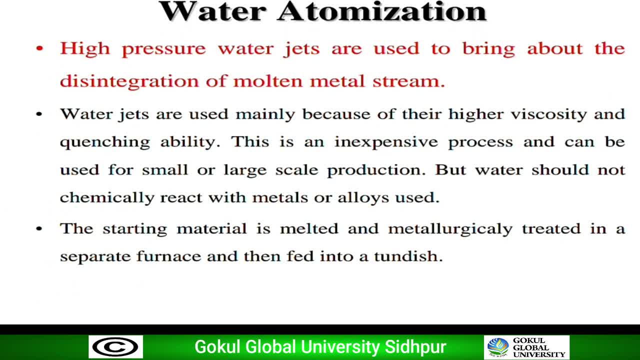 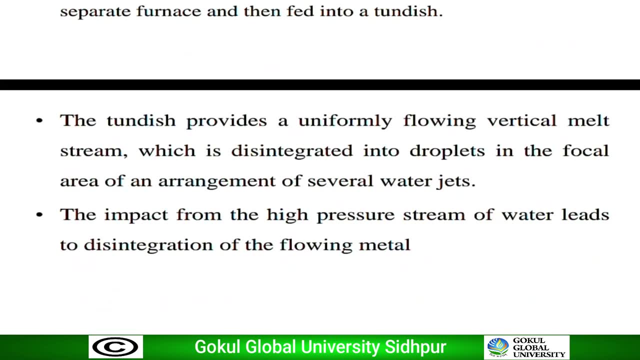 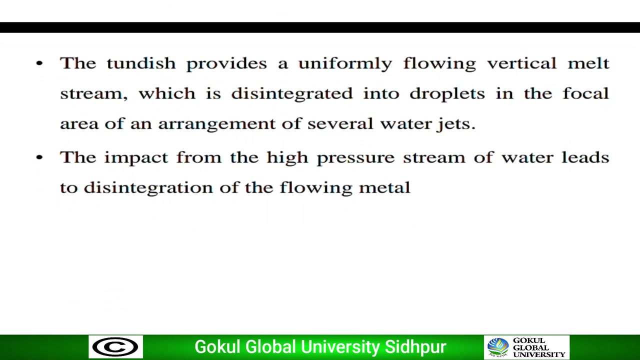 used. the starting materials is melted and metallurgical treated in separate furnace and then feed into tundish. now what is the discuss about? to this? tundish provide a uniformly flowing, vertically melt streaming which is distingrated into droplets in the focal area of an. 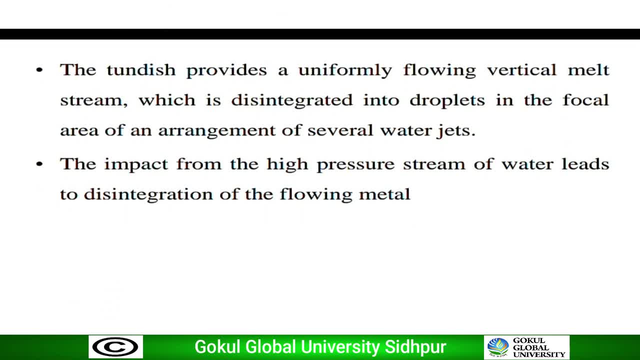 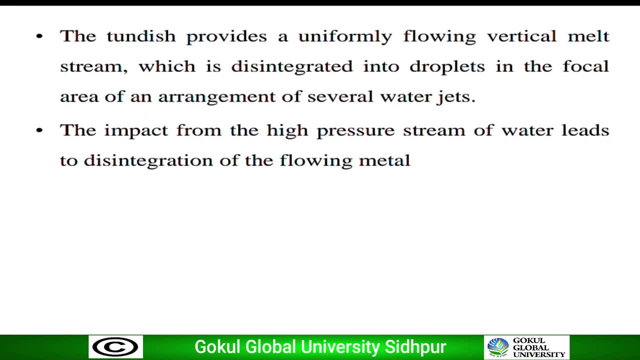 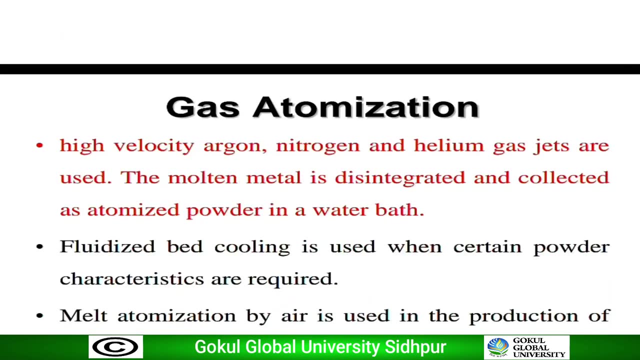 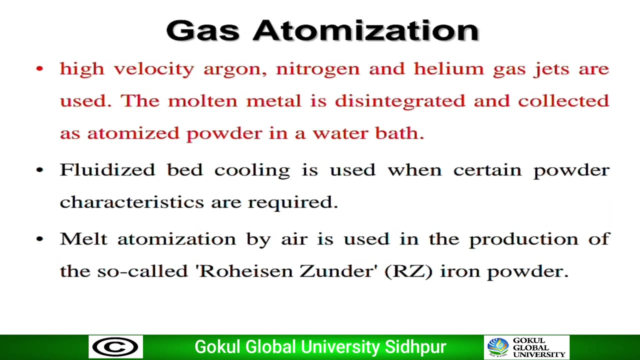 arrangement of several water jets. the impact from the higher pressure stream of water lead to distingration of flowing metal. now friends discuss about a gas atomizations. now gas atomizations, high-velocity argon, nitrogen and helium gas jets are used. the molten metal is distigrated and collected as atomized powder in the 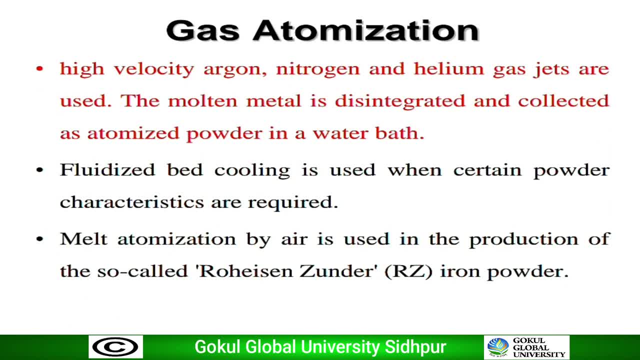 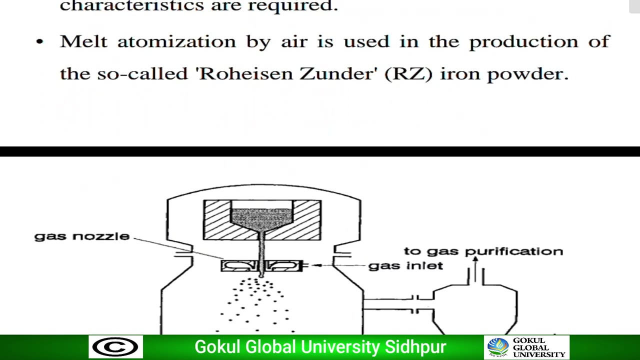 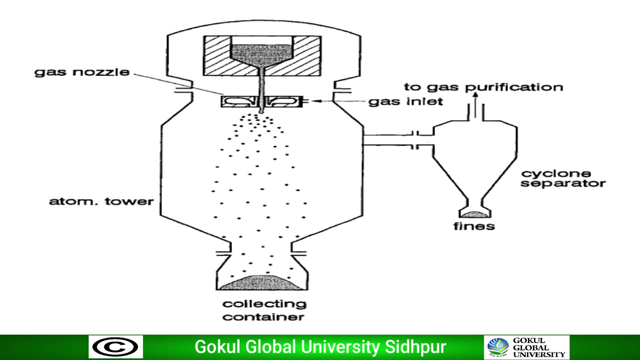 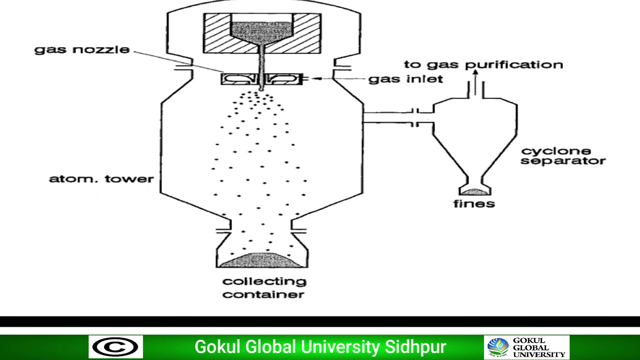 water bath. fluidized bed cooling is used when certain powder characteristics are required. melt atomization process is used to bring about the distinctions of molten metal stream and underground. underground vaporization process. now enter the Hoper in various types of gaseous flowing with waters. substance with a gaseous now 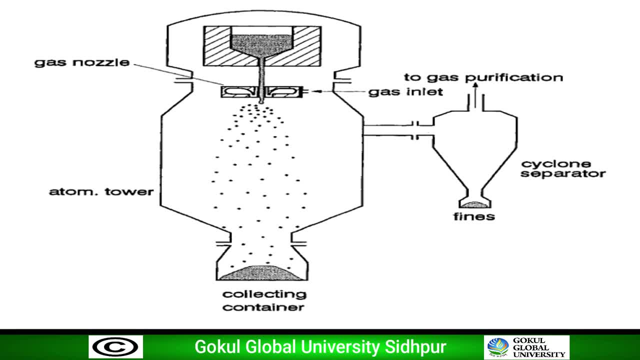 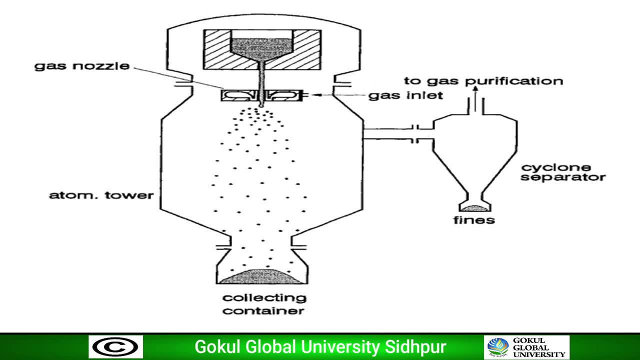 second one is gaseous Saros. också antiprewertified cokin sẽ hôp 안에. reunion of organic gas strategies across the inlet and collecting containers: collect with abrasive particles small abrasive abrasive particles. then atomization tower collect the various types of vapor. 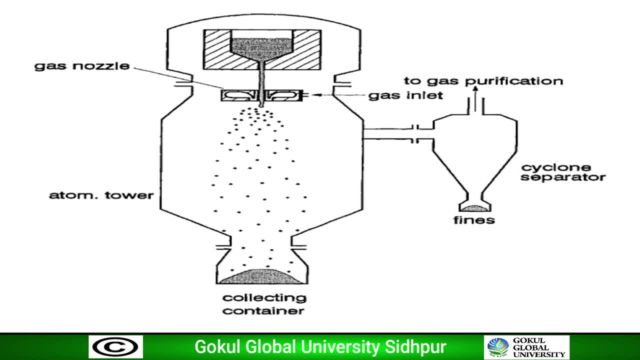 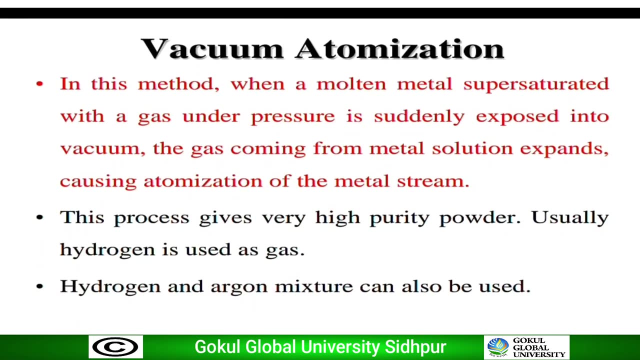 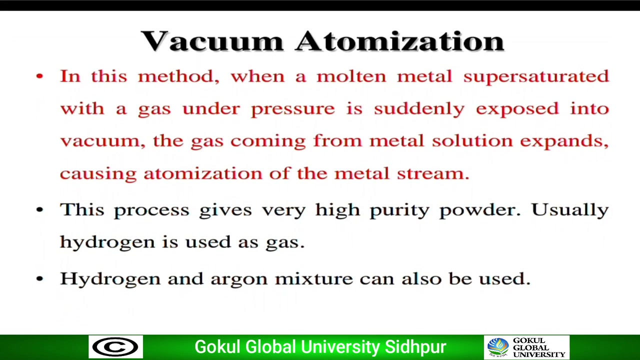 with the gaseous, then cyclone separators collect the fines vapors and these purified gaseous. now friends discuss about a vacuum atomization in this method, when a molten metal, super saturated gas with the gas under pressure is suddenly exposed into vacuum, the gas coming from metal solution. 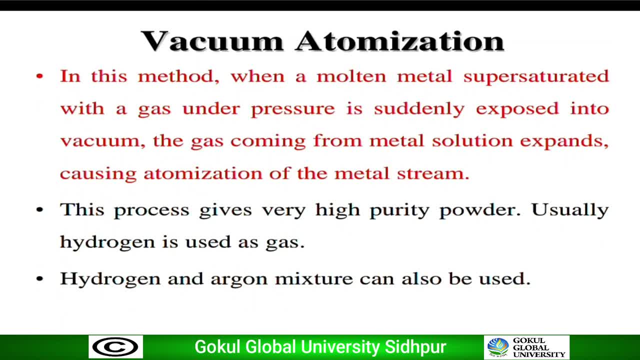 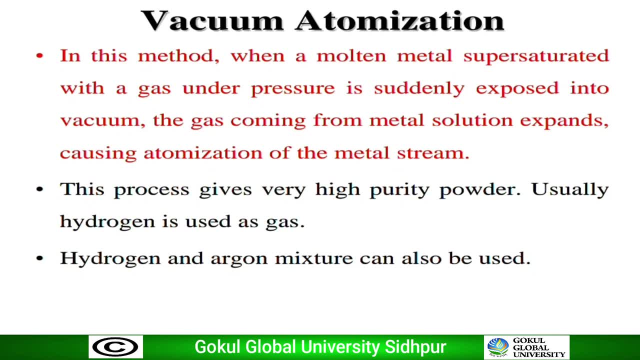 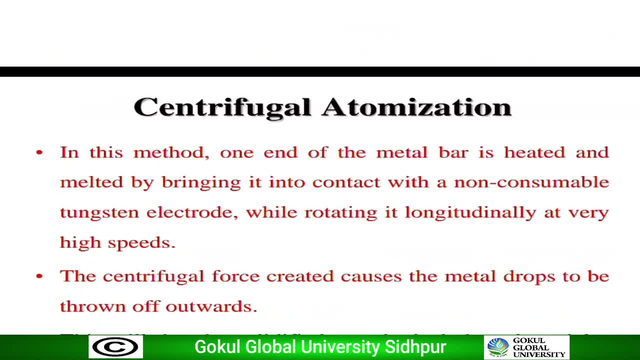 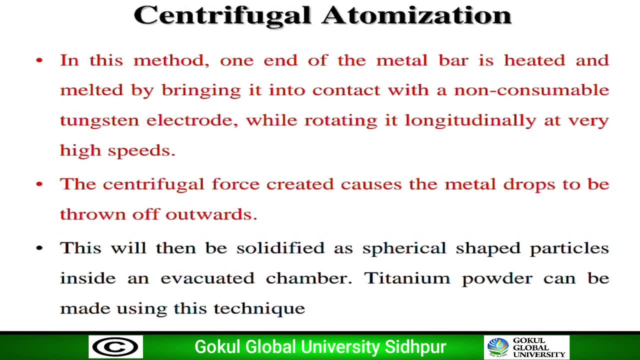 now friends discuss about centrifugal atomizations. in this method, one end of the metal bar is heated and melted. by bringing it into to contact with a non-consumable tungsten electrode like that Tig welding, while rotating it longitudinally at very high speeds, a centrifugal force create. 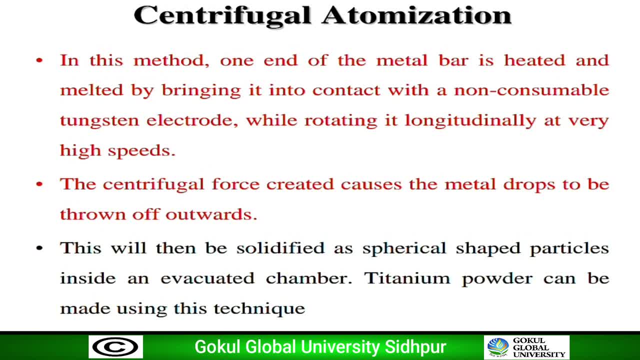 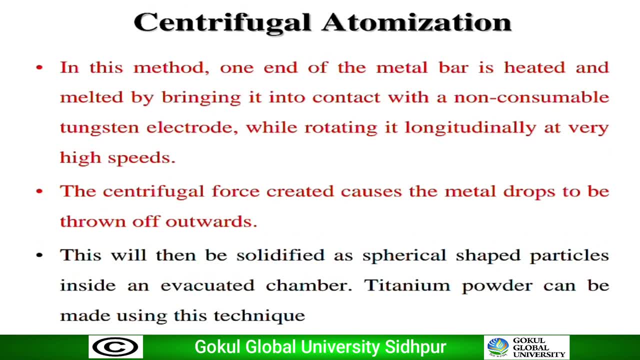 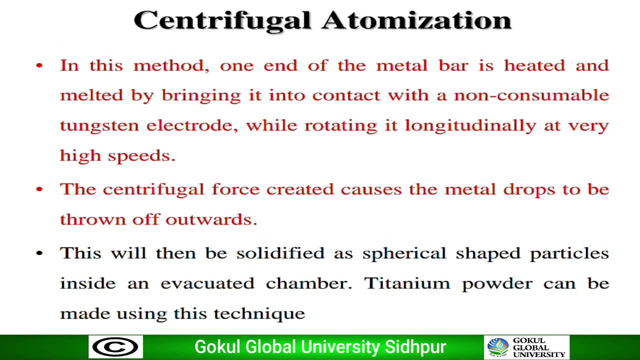 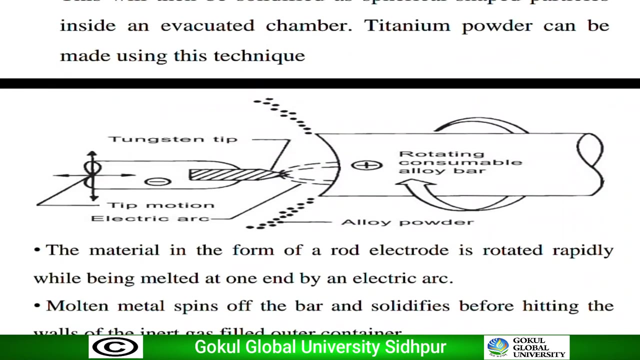 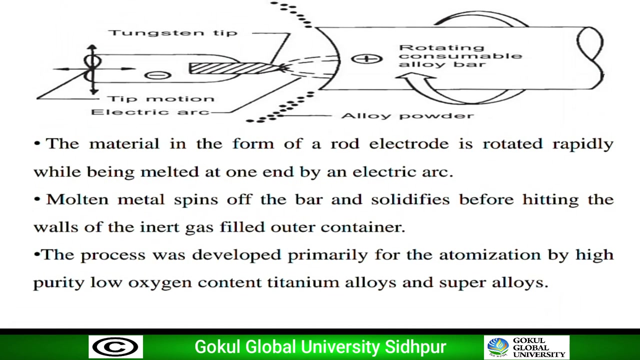 causes the metal drops to be thrown of outwards. this will then be solidified as spherical, safe particles inside evacuated chamber. like that, titanium powder can be made using these techniques. now, friends, see this figure. the material in the form of a rolled electrode is rotated rapidly while being 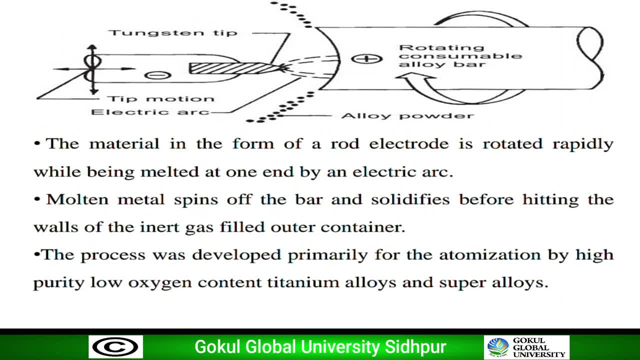 melted at one end by an electric arc, the material in the form of a rolled electrode is rotated rapidly. while being melted at one end by an electric arc, the molten metal spins of the bar and solidifies the. before heating, the falls of the inert gas filled outer containers. this process was developed. 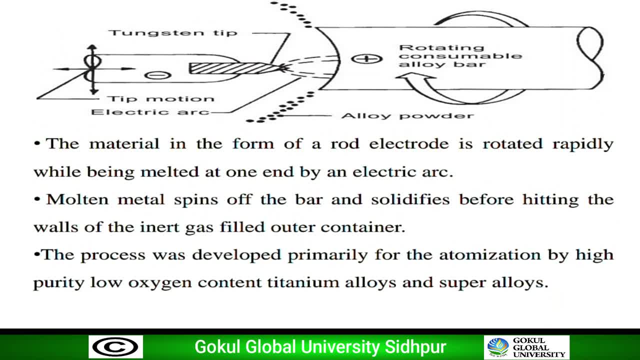 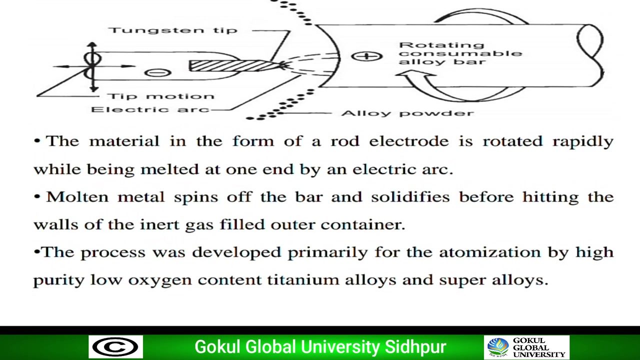 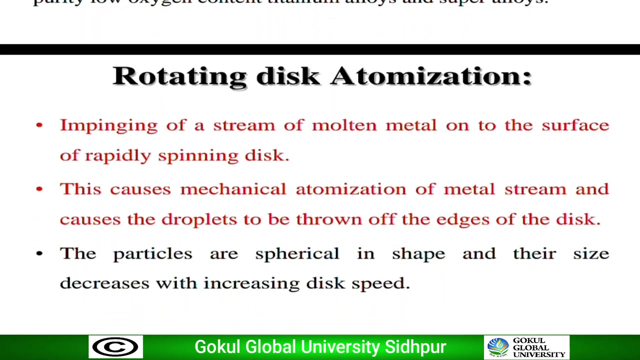 primarily for atomization by high purity. now discuss a rotating bar. this is a rotating bar: is the plus container and your tungsten tip is the negative. this is the process. was developed primarily for the atomizations by high purity, low oxygen, contain titanium alloy and super alloys. now friends discuss about rotating disk atomizations. 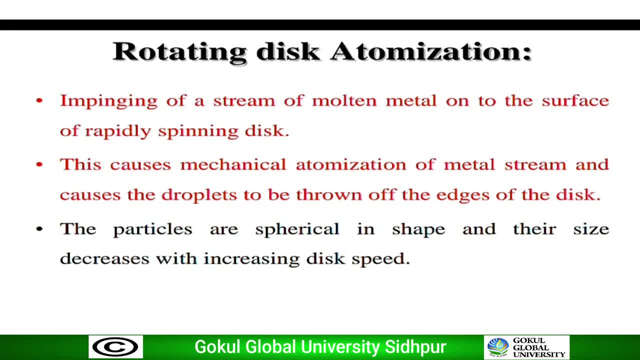 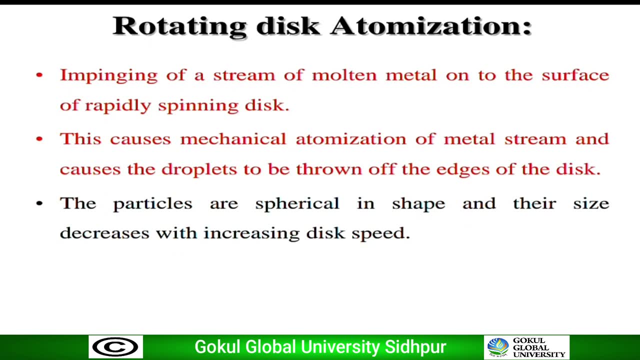 imping of a stream of molten metal on to the surface of rapidly spinning disk. this causes mechanical atomizations of metal stream and causes the droplets to be thrown of the edges of the disk. the particles are spherical in the shape and their size decrease with increase in the size of the disk. 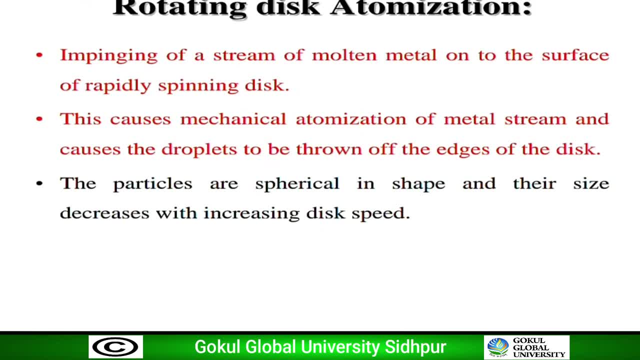 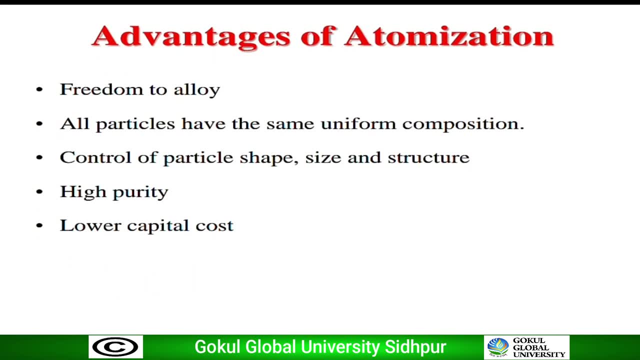 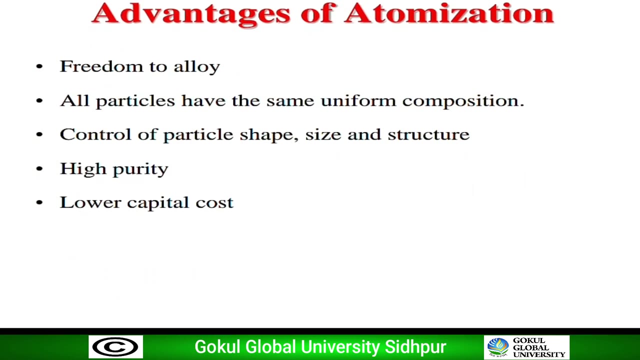 increasing disk speed. now, friends are discussed about advantages of atomizations: freedom to alloys. second, and all particles have same uniform compositions. third, one is control of particle shape, size and structures: high purity, lower capital cost. now discuss about a heat treatment of powders. now, what is the heat treatment of powders now? what is the heat treatment of powders? 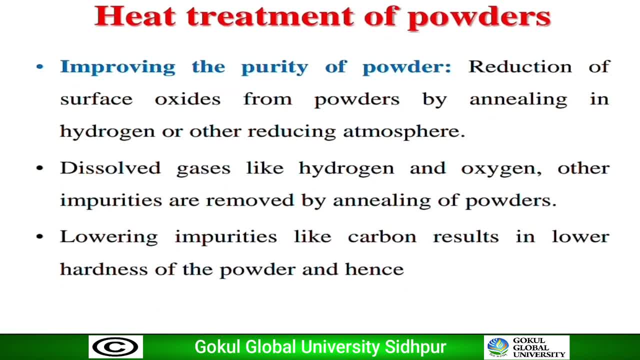 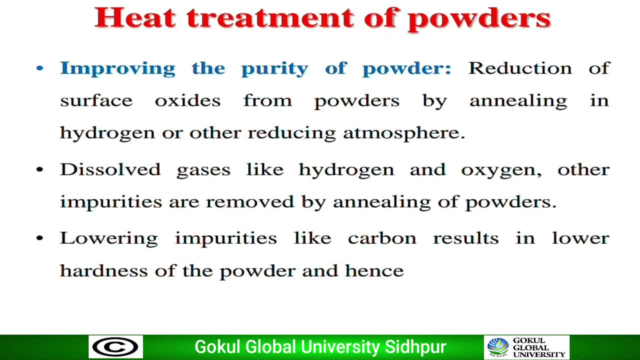 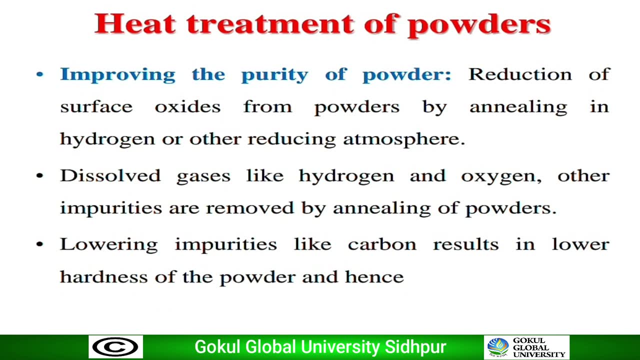 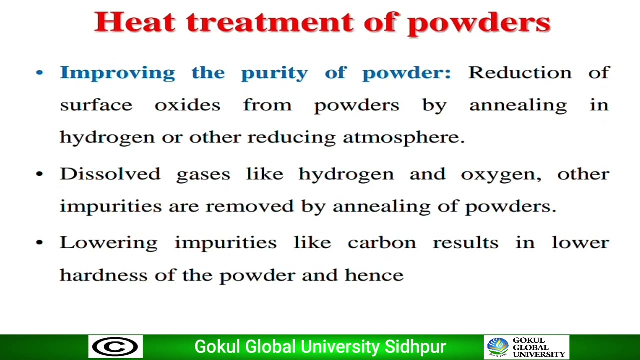 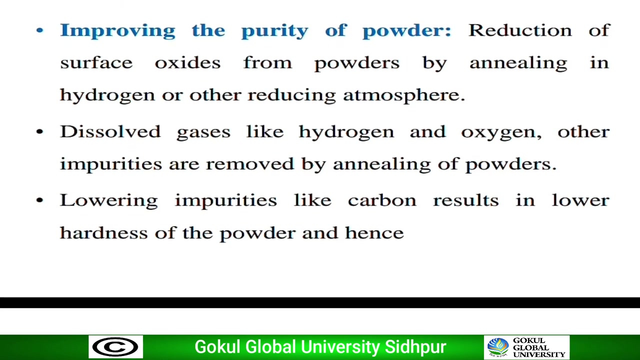 the first one is improving the purity of powders: reduction of surface oxide from the powders by annealing in hydrogen or other reducing atom atmosphere now dissolved gaseous like hydrogen and oxygens. other impurities are removed by annealing of powders. lowering impurities like carbon results in lower hardness of powder and hence 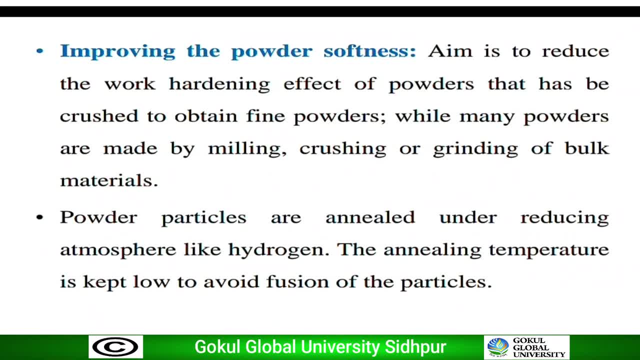 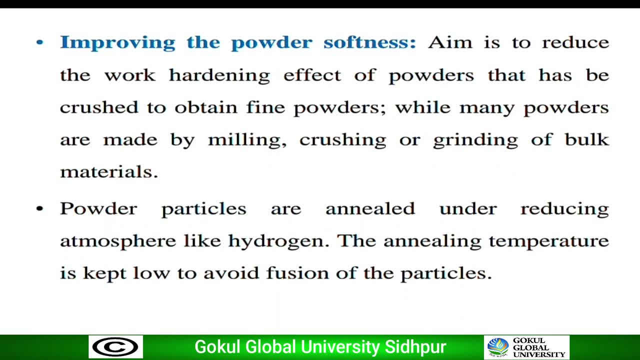 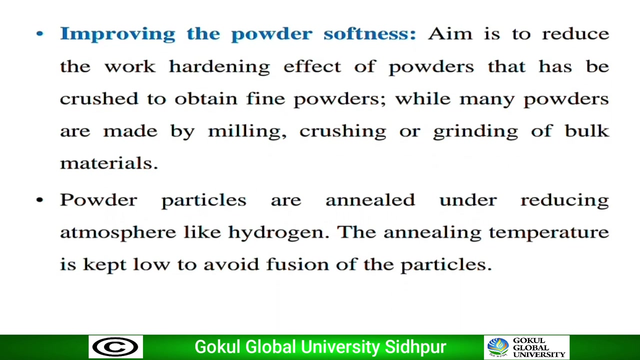 second one is improving the powder softness. now, what is the powder softness aim to? to reduce the work hardening effect of the powders that has been crushed to obtain fine powder. while many powders are made by milling, crushing or grinding of bulk materials, powder particles are annealed under reducing atmosphere, like hydrogen. 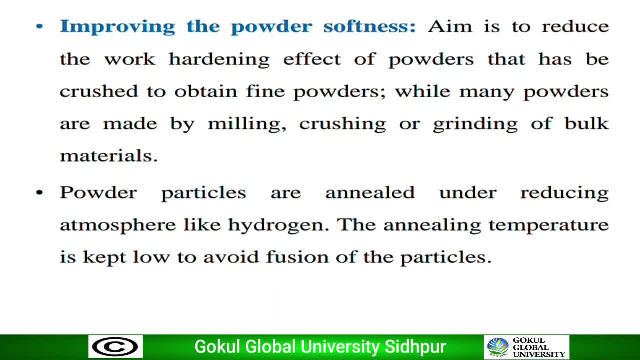 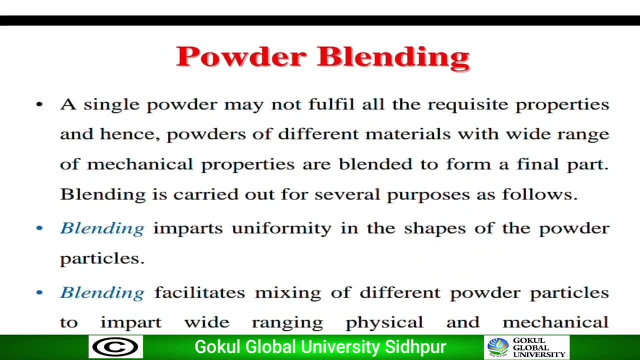 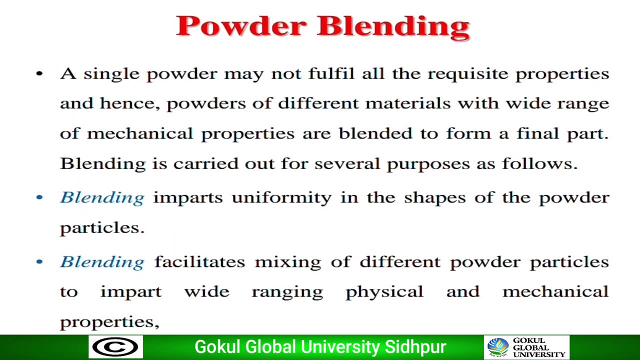 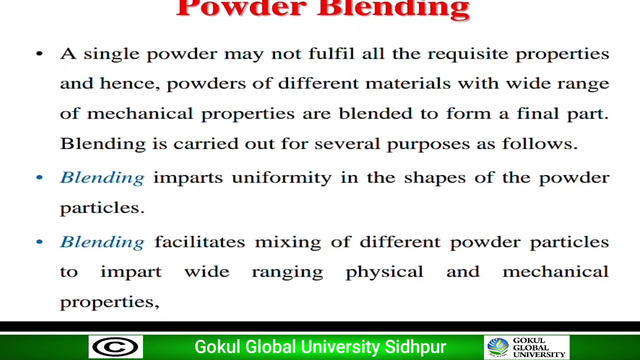 the annealing temperature is kept low to avoid fusion of the particles. now next process: powder blending. Now, friends, powder blending is the one type of single powder may not fulfill all the required time properties and hence the powder of different materials with wide range of mechanical properties are blended to form a final parts. 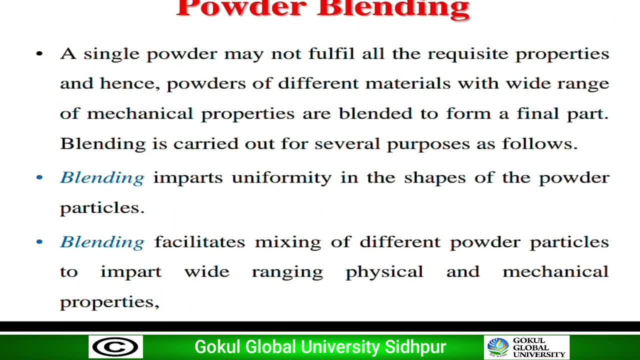 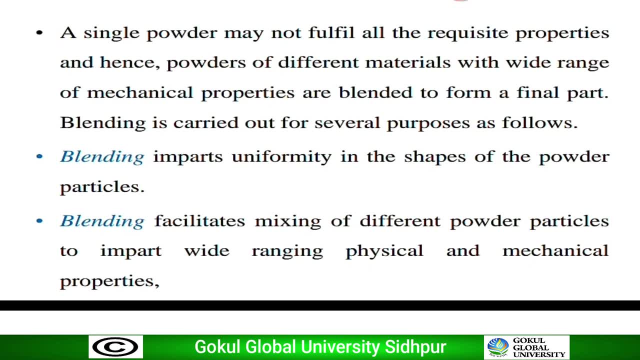 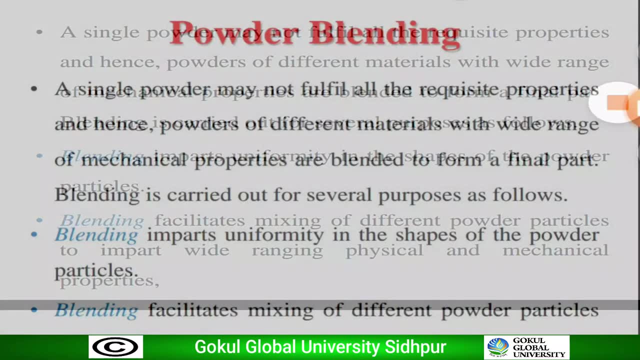 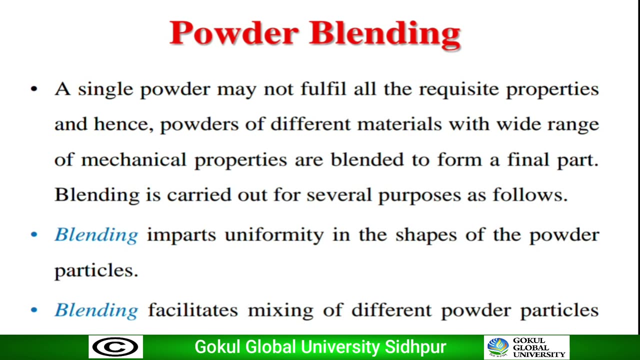 Blending is the carried out for several purposes has followed Now. first one is blending. Blending is the impart uniformly in the shape of powder particles. Now friends discuss about a powder blending process. Now, powder blending is the one type of. is the obtain a homogeneous mixture. 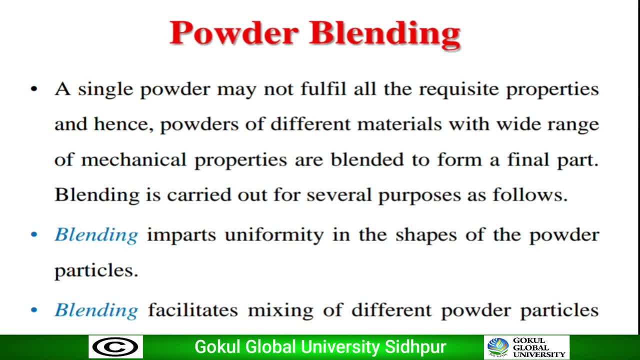 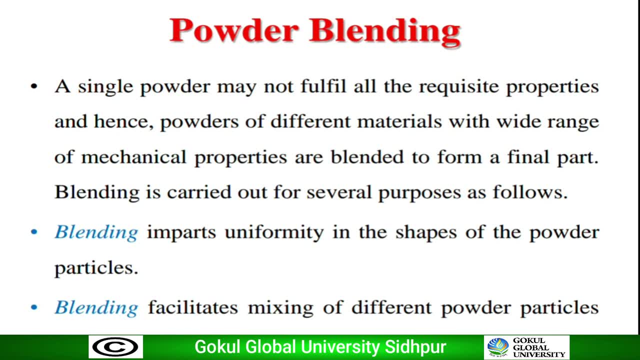 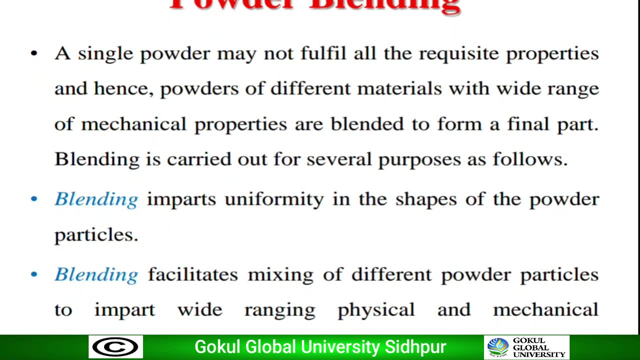 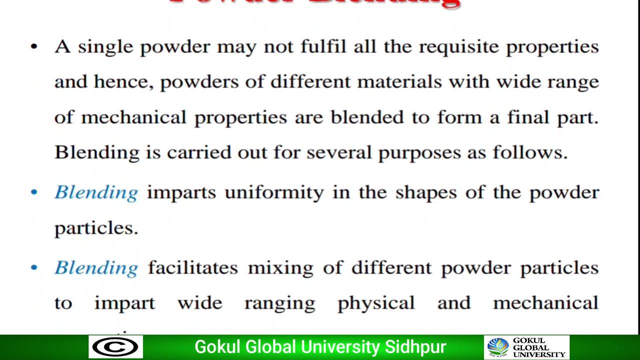 of powders and improve the compacting and sintering properties In this process, through mixing of powders of some materials or different material is in corn. Now a single powder may be not fulfill all the required time properties and hence powders of different materials. 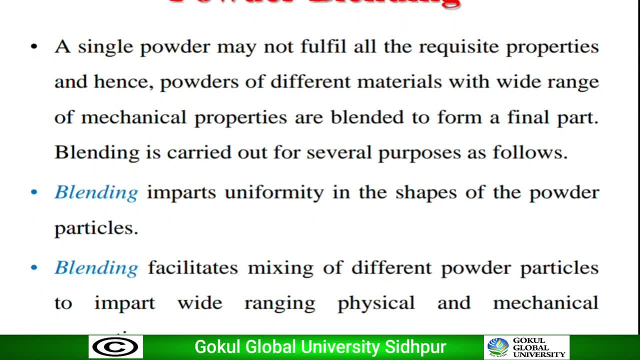 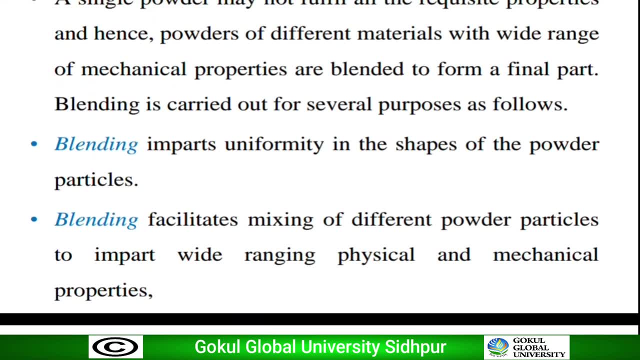 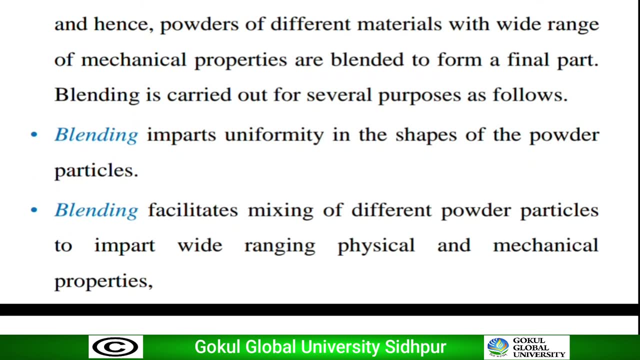 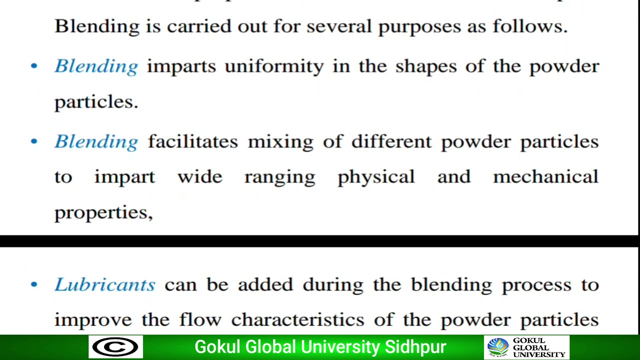 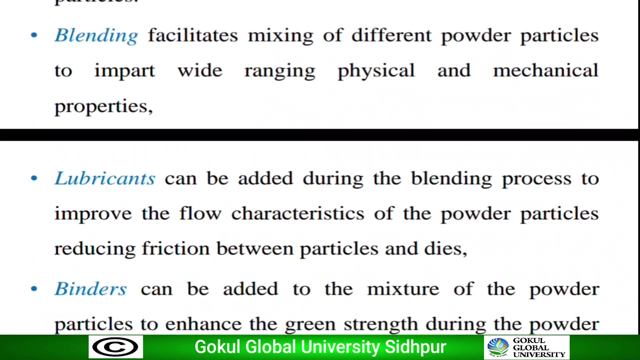 With wide range of mechanical properties are blended to form a final part Now blending. Blending is the impart uniformly in shapes of powder particles. Blending is the facilitated mixing of different powder particles to impart wide-ranging physical and mechanical properties. Now discuss about lubricant. 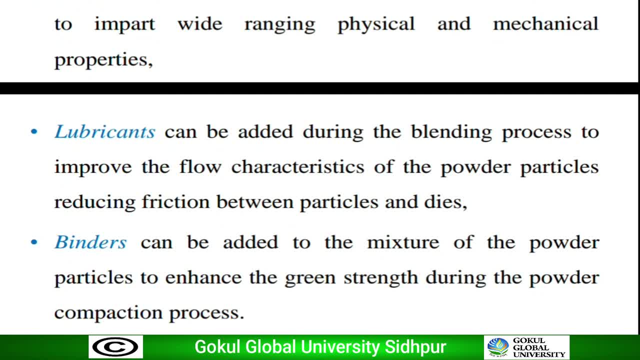 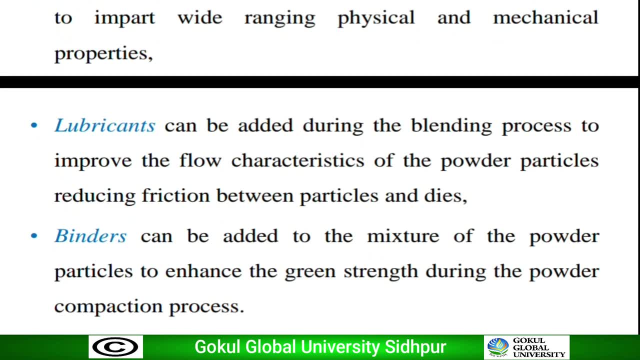 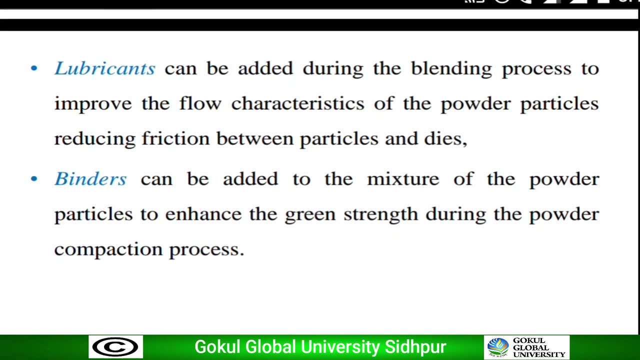 Lubricant can be added during the blending process to improve the flow characterized of the powder particles, Reducing friction between particles and dyes. Now a binders Binders can be added to the mixture of powder particles to enhance the grain strength during the powder compactions of process. 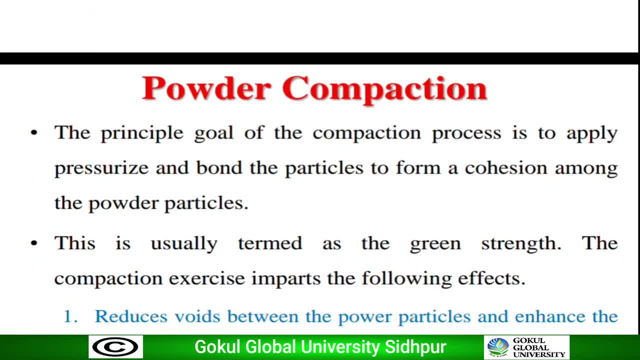 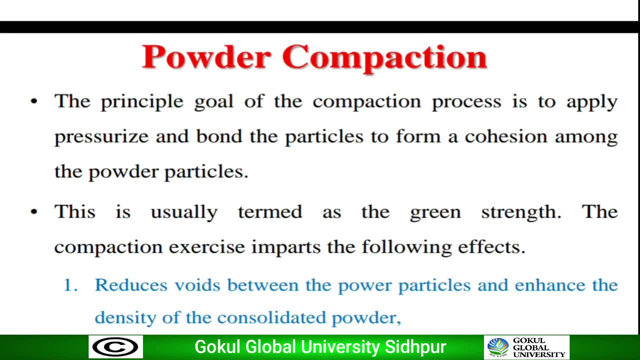 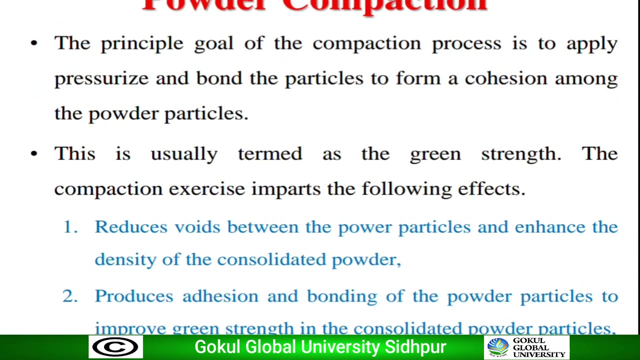 Now discuss about a powder compaction. This principle goal of compaction process is to apply, pressurize and bond the particles to form cohesion. among the powder particles This is usually terms as the grain strength. The compaction exercise impart the following effects: 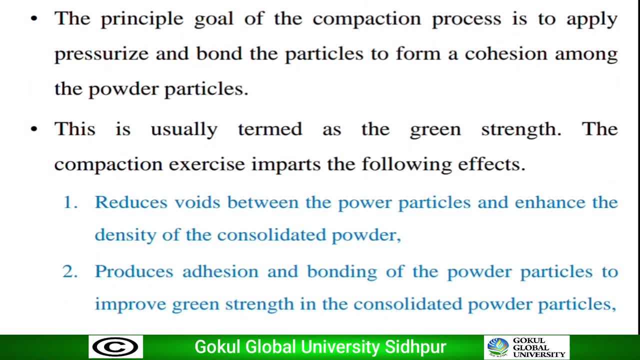 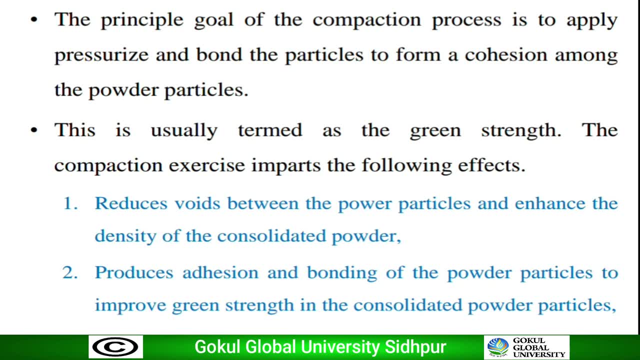 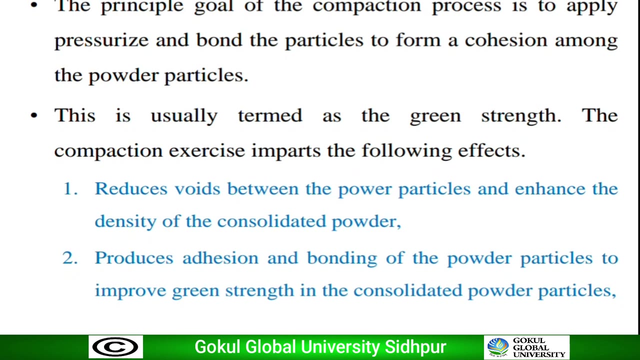 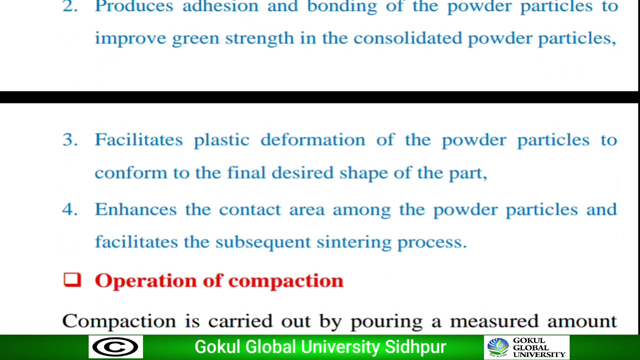 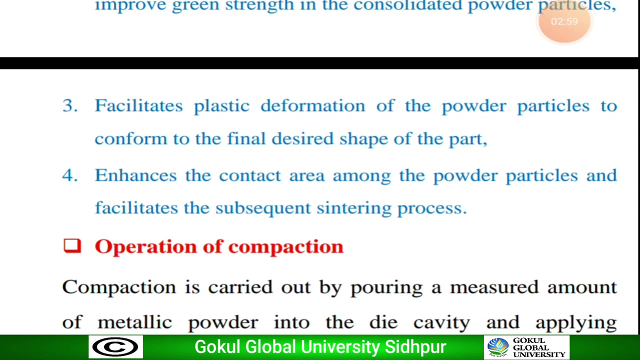 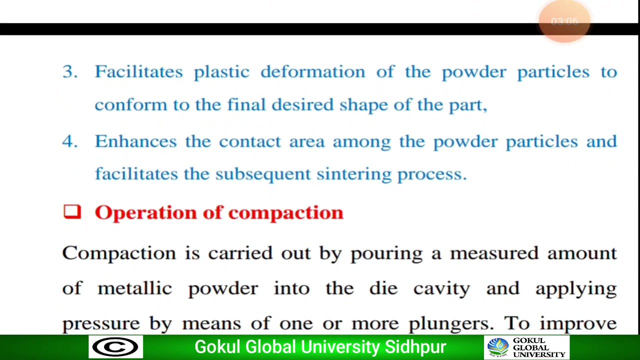 Now, first one is reduce void between the powder particles and enhance the density of consolidated powders. Second one is produces addition and bonding of powder particles to improve grain strength in the consolidated powder particles. Now third one is facilitate. Third one is facilitates plastic deformation of the powder particles to conform to the final desired shape of the part. 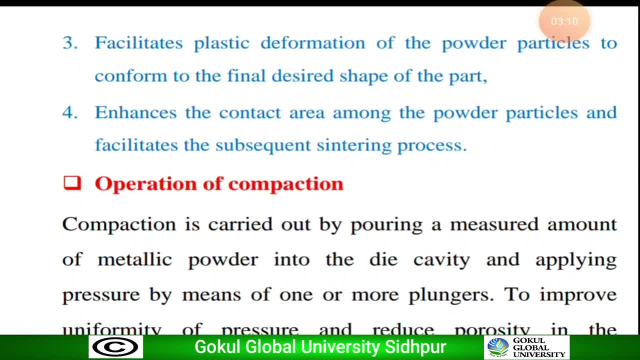 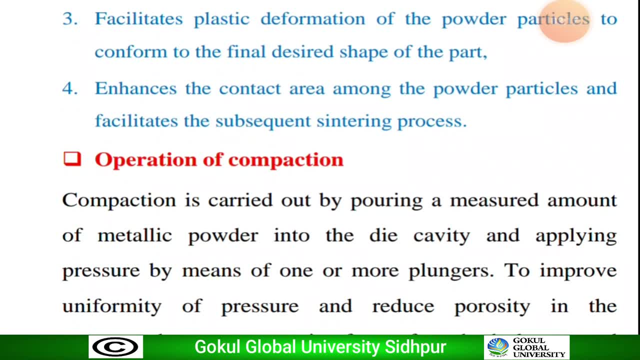 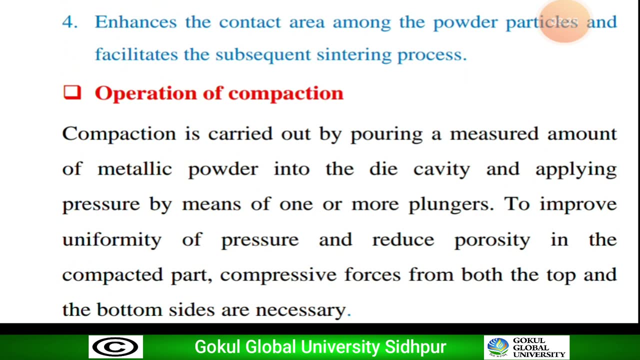 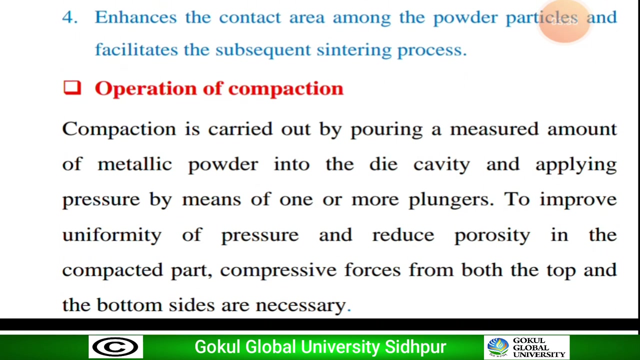 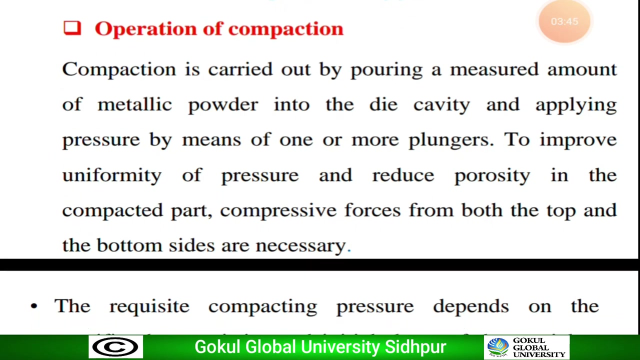 Fourth one: enhance the contact area among the powder particles and facilitate the subsequent sintering process. Now, operation of compactions. Compaction is carried out by pouring measured amount of metallic powder into the die cavity and applying pressure by means of one or more plungers to improve uniformity of pressure and reduce porosity in the compacted part. 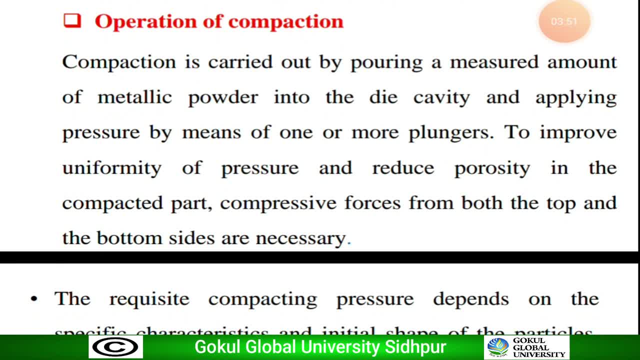 Now the final step is to apply and then to compress. Compaction of powder and difficult compressive forces from both the top and bottom sides are necessary. Now discuss what is the compound compounding pressure. Now discuss what is the compound compounding pressure. 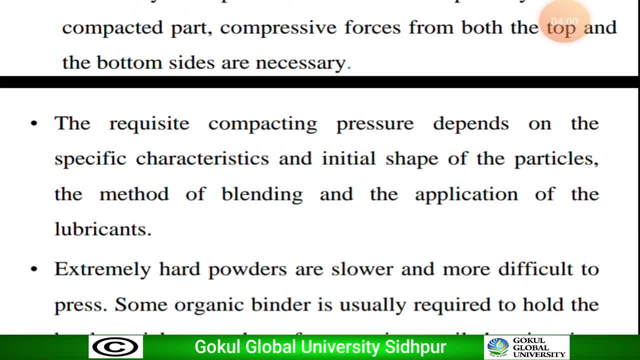 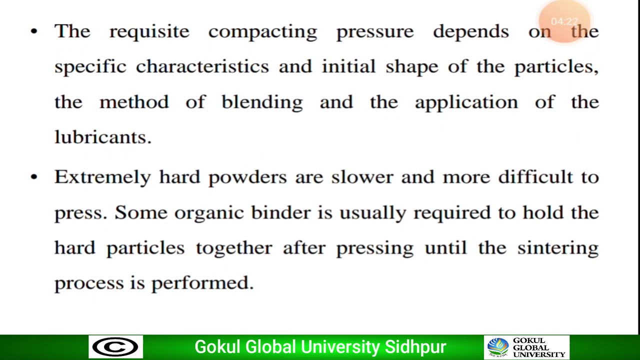 Now discuss what is the compound compounding pressure? This request side. compacting pressure depends on the specific characteristics and initial shape of the particles, the method of blending and the application of lubricant. Extremely hard powders are slower and more difficult to press. 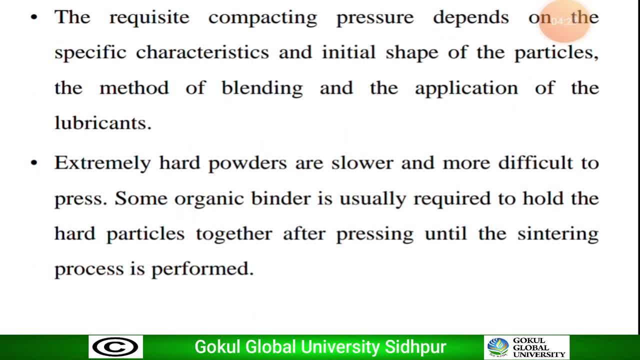 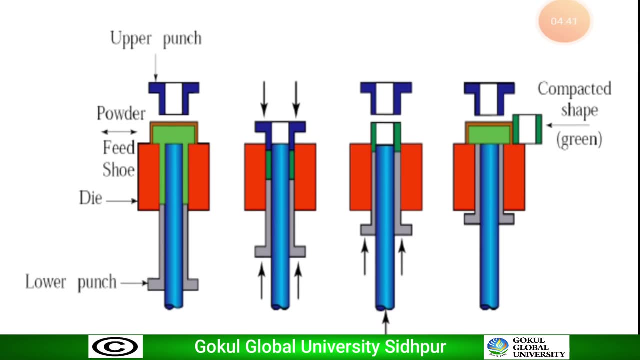 Some organic binder is usually required to hold the hard particles together after pressing until the sintering process is performed. Now this is the figure of compaction. The upper punch is pressing and powder should die. Then lower punch is push out. Then second stage. 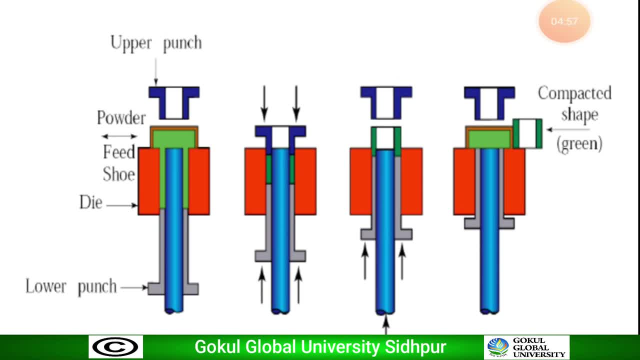 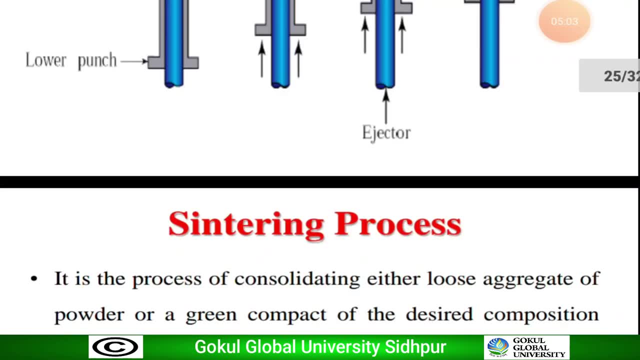 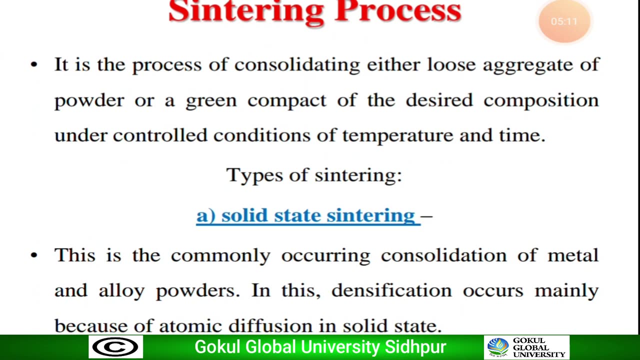 The lower punch is: push out to die. And finally is the compacted shape. It's the green color. Then next discuss about sintering process. It is the process of: 1. Consolidating either loose aggregated of powder or green compact of the desired composition. 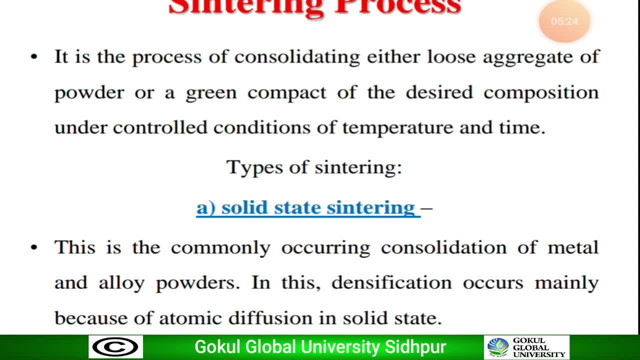 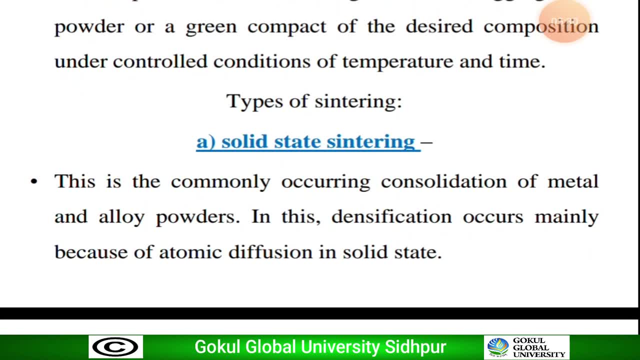 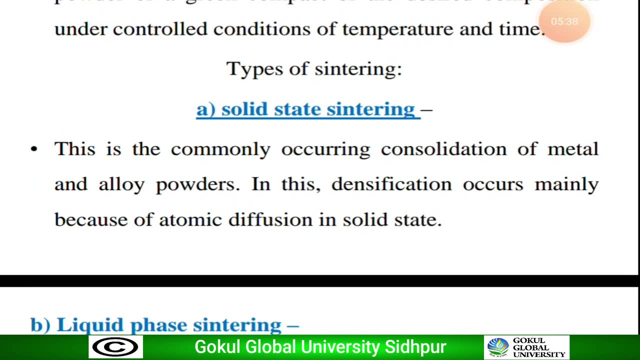 under control conditions of temperature and time. The types of sintering process: Solid state sintering process: This is commonly occurring. consolidating of metal and alloy powders. In this Densifications occur mainly because of atomic diffusions in solid state. 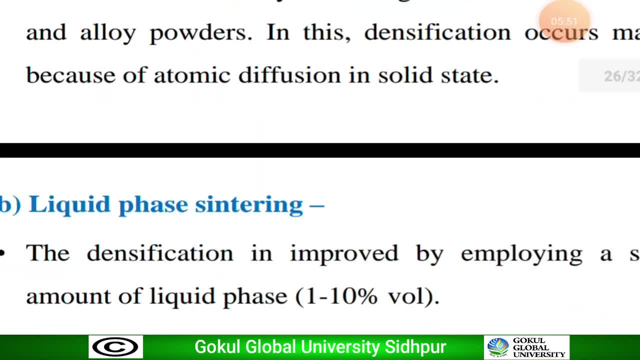 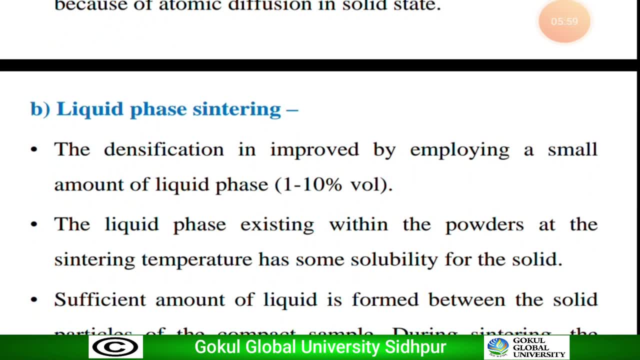 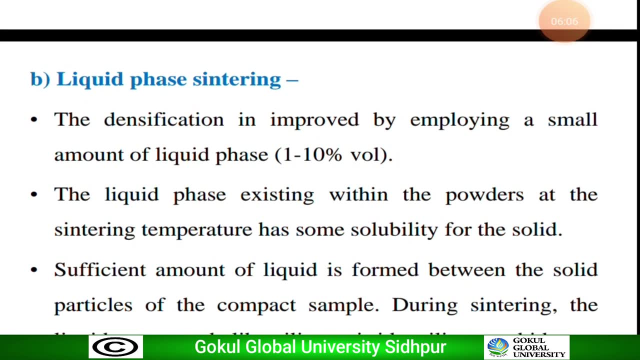 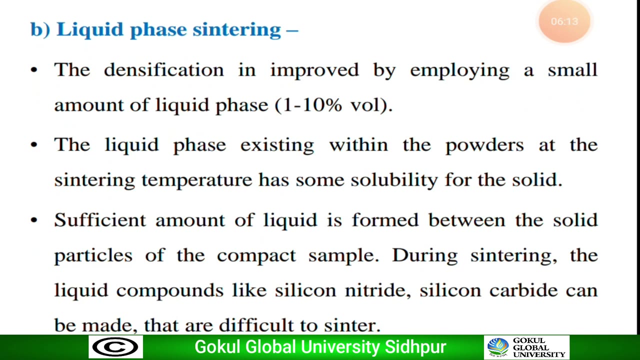 Then second one is Liquid phase sintering process. The densifications in improve by employing a small amount of liquid phase 1 to 10% volume. The liquid phase exciting within the powders. 2. At the sintering temperature has some solubility of the solid. 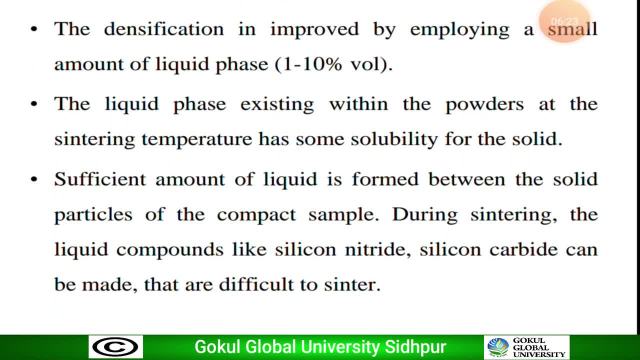 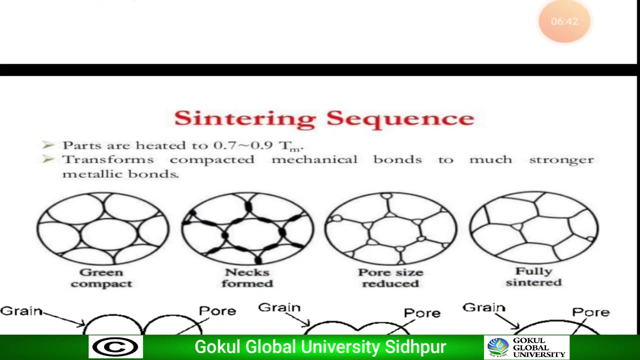 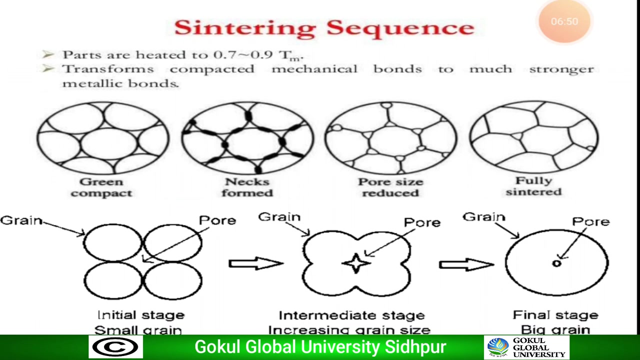 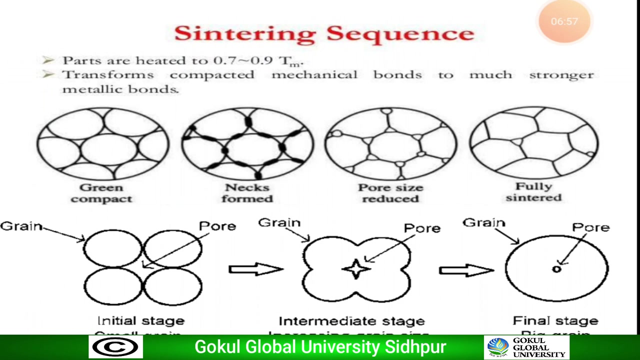 Sufficient amount of the liquid is formed between the solid particles of the compact sample. 3. During sintering, the liquid compound, like silicon nitride, silicon carbide, can be made that are difficult to sintering. 4. Daily. 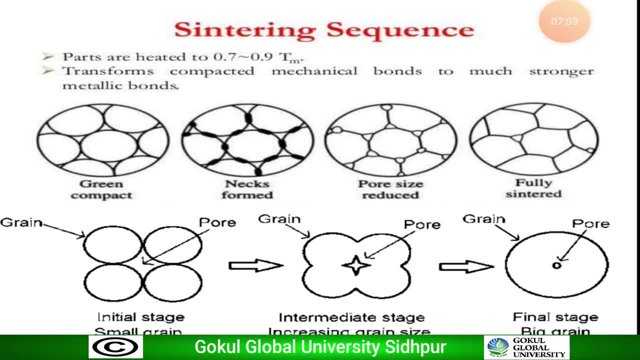 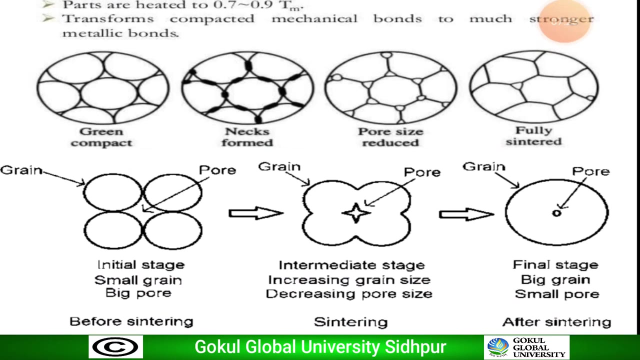 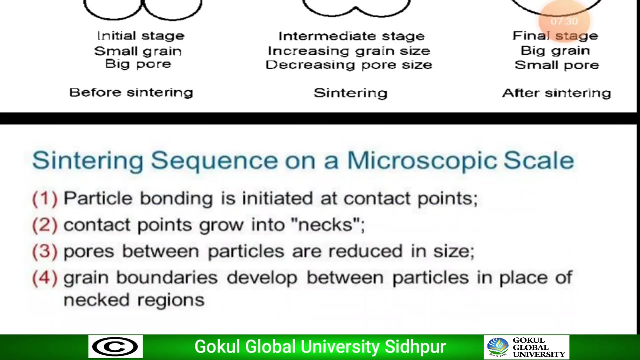 5. of atoms, and it's diffused and destroyed to pure size, reduce and finalize fully sintered. this is the diagram of before sintering process and after in sintering process, sintering sequence on a microscopic scale. first one is particle. 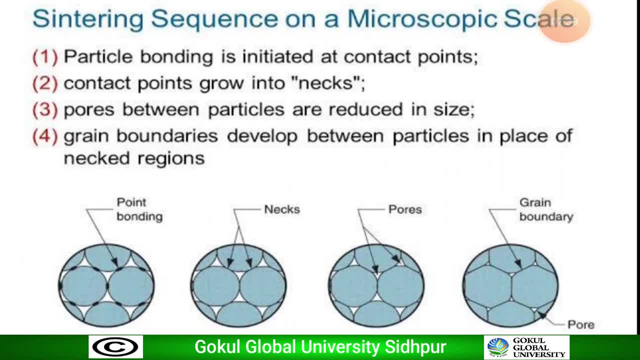 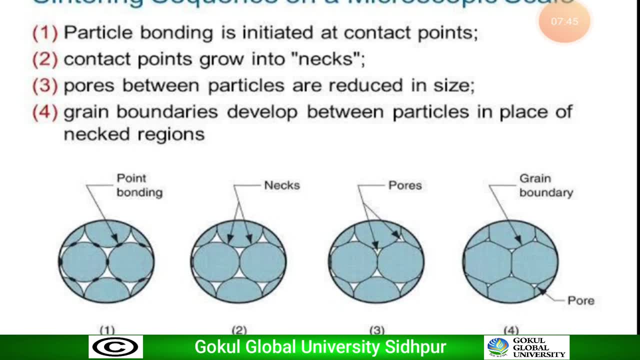 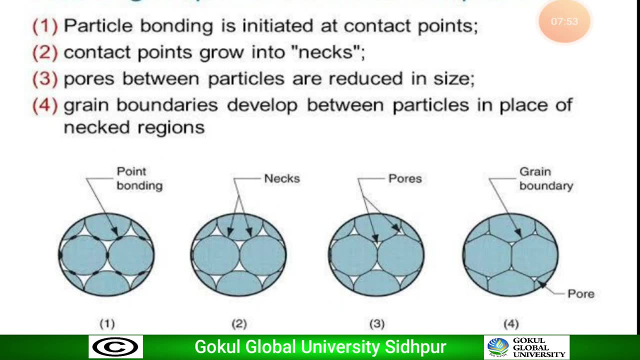 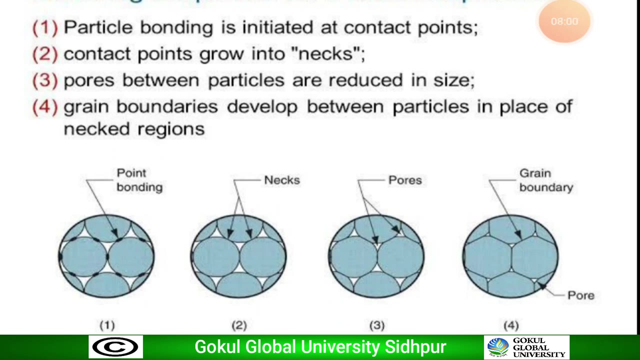 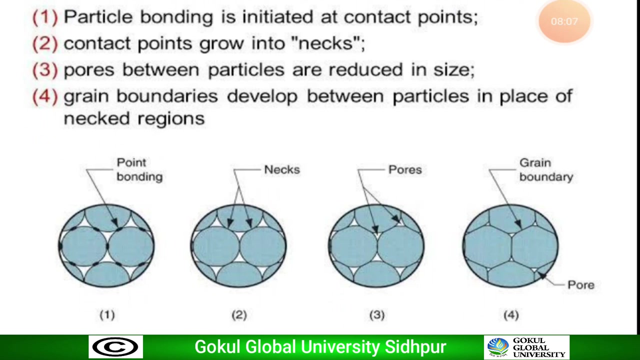 bonding is immediate at content points. now, second one is contact point. grow into neck neck means atoms will be destroyed and can be converted into small particles and small particles it's again destroyed and pores between particles are reduced in size. then, after finalize, grain boundaries developed between particles in place of 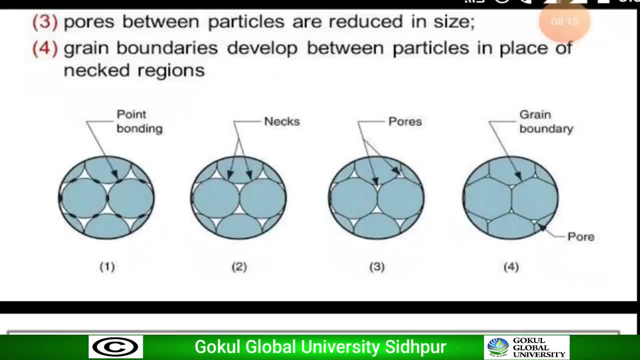 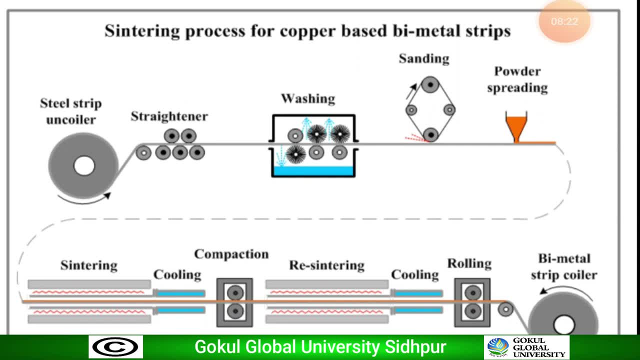 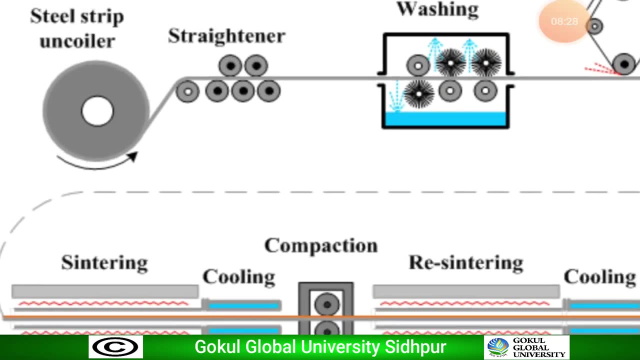 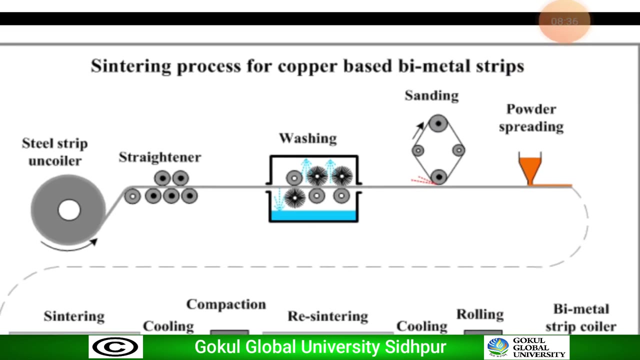 neck regions. now, friends, this is the example of sintering process of copper base b-metal strips. this is the first one is steel strip uncoiler. it's converted into straightener. it's a pressing different types of roller. then after it's going in the washing section, washing.